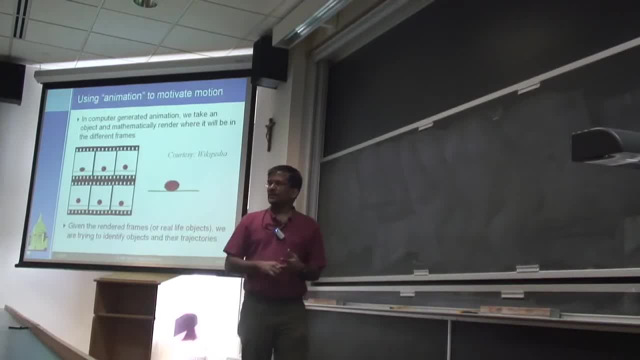 to achieve and why it's so hard to do the compression right. So, animation, we are going into the detail right. In the simple form you kind of create some sort of object right, And the more complex the object is, the more realistic it looks and all those things, But in the simple. 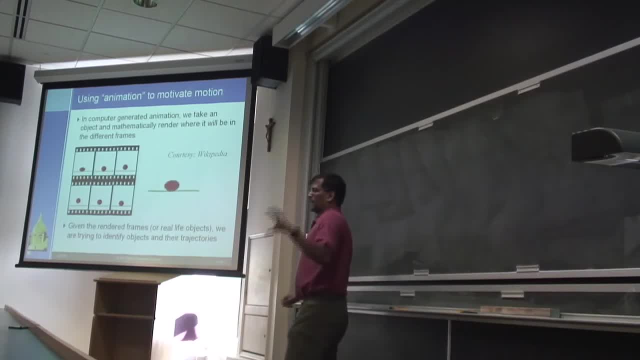 form. you take some object and if you want to animate, you kind of figure out where this object would be at different points in time. So if you're going to do a 30 frames per second, you decide where it will be in the 1, 30th of a second, next 1, 30th of a second, and so on, using some sort of 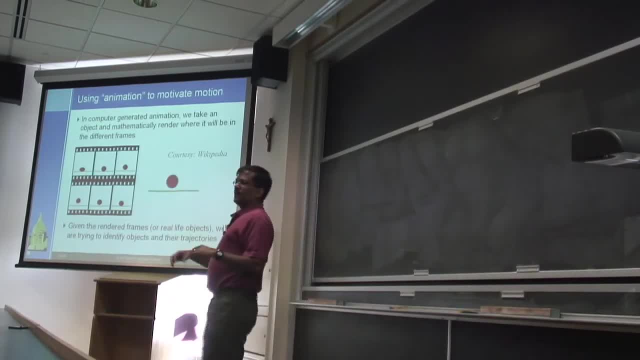 some calculation right. So if you're looking at a bouncing ball, you have a notion of the ball, you know the weight of the ball and the gravity and all those things to decide where this thing should be right. So you may decide that this ball starts off here. 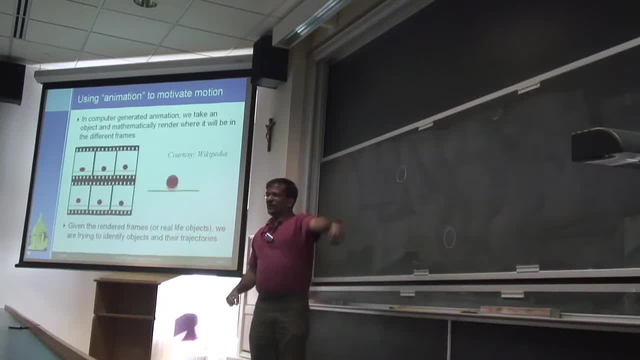 and one second. it's going to be here, right. So you have to have some kind of equation which figures out that it's going to take this trajectory, right. So you say in the frame 1, it will be this, frame 2, this will be this, frame 3 will be this, this, and so on and so forth. 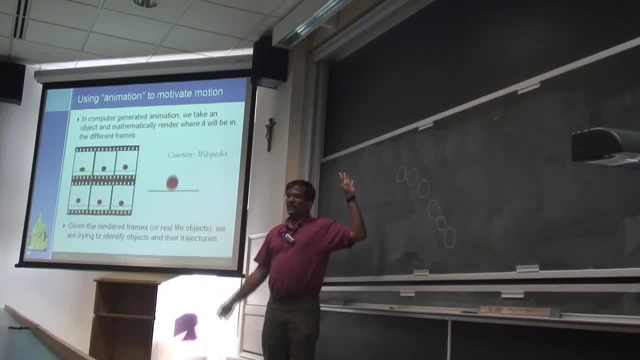 right, And if you play it at the same time, you have a notion of the ball. you know the weight of the rate that you are looking for. it looks like it's moving even though it's going here. So I think I got the Wikipedia. so you see those little sequences and when they're played at a 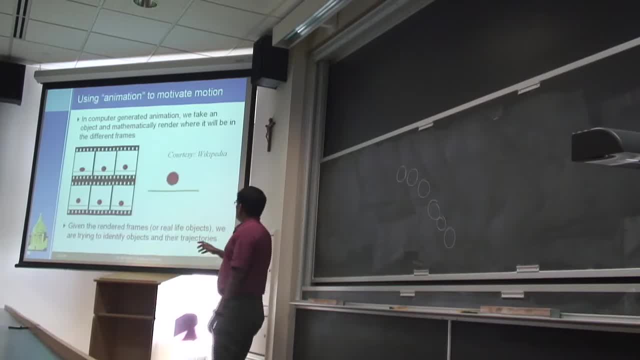 certain rate, it looks like the ball is bouncing right. There are more issues. I mean they make the ball kind of squish and all those things ignore those aspects, right? So what you're trying to do is the compression form. we don't know that there's object, right? We don't know. 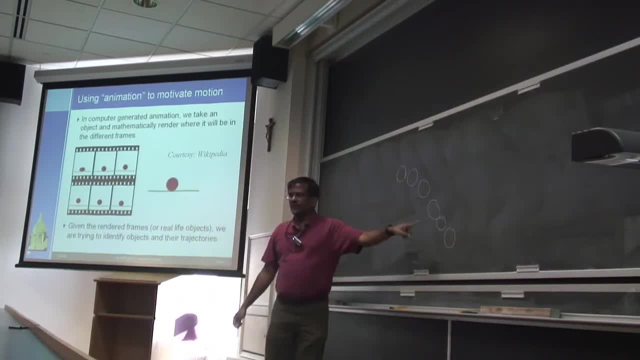 what this trajectory and all those things. we would like to look at these individual frames, right, And sort of predict what is happening, right. So then we could basically say: draw this one and the next one is a simple translation from here to here, even though in the real animation, 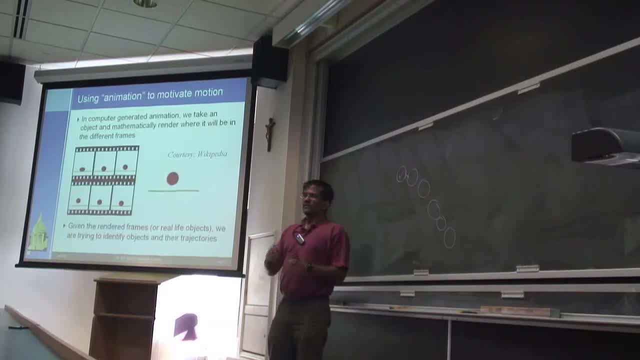 case, it's not a simple like linear transformation, it's actually going to some sort of a more complex equation, right? So we would like to say: from here, the next one should be: you know this, far from here, and take this one, go from here, go from here, and so on and so forth. right, So I take the. 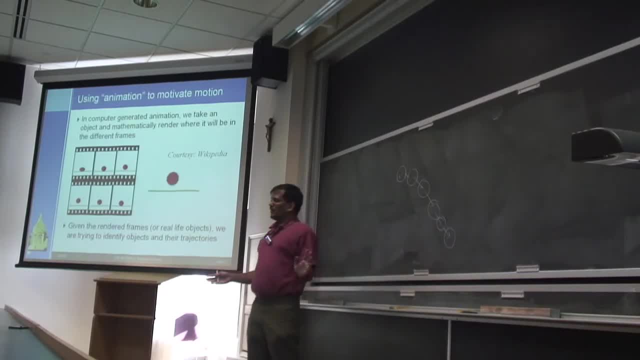 first one. then I kind of try to predict this stuff right. If that's all I have to do, it's far trivial. The real case is we are looking at a real scene where there's a more complex object, not a circle kind of thing. So I need to figure out what is the object in a frame, right? So if you look at 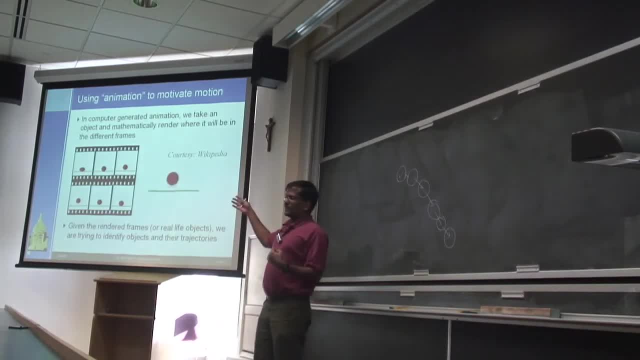 this scene I'm standing here. I'm more complex than a round ball, So you have to figure out where my object is and you have to figure out where I would have moved right. So you're trying to figure out what these things are on a complex scene. So you have to figure out where my object is and you 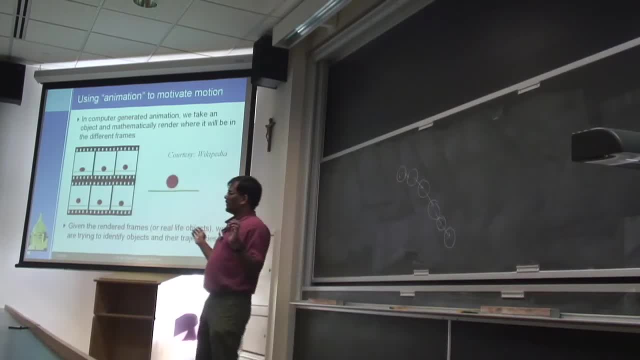 can see complex objects which are moving in different ways, in completely unpredictable ways, right? So it could be like saying something very close to you. it could be something very far. So you're trying to figure out what this is. If you can do something about it, you get good compression. 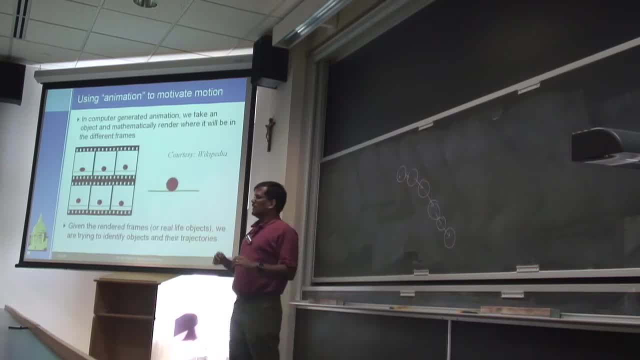 If you can figure out how these motions were, you can get good compression. If you can't, then you don't get any compression right. So the goal is: there are some algorithms which go through the scene. So if you have a 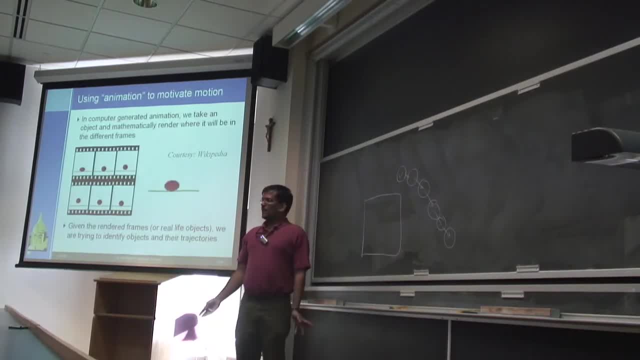 image. I have no idea what objects are and what they are moving. so I am going to start from this image I am going to look at. let's say so. I have the target and the reference and if you take the reference as the previous one and the target as the current one, if 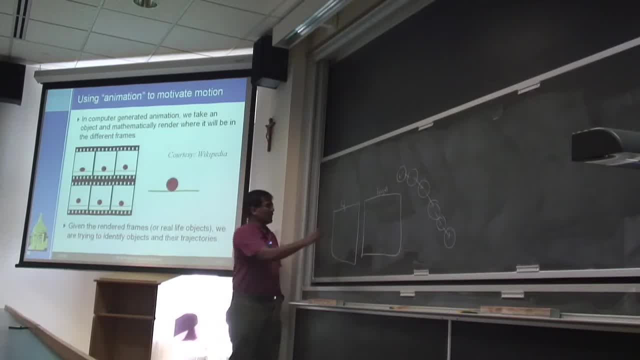 you are taking these two frames. I have to go through here in some way. sweep through this stuff. if it is a simple animation like this, I am going to look at all the objects which are here and see where they moved over here this. I have no notion of objects and 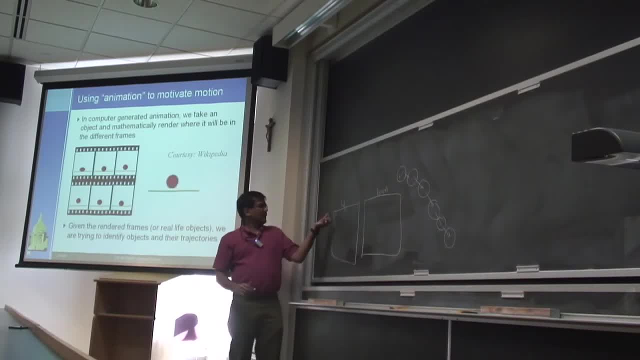 stuff. I am going to look at each one of these things, right. so I am going to take this particular square and I am going to see where this square might have moved, right, And I am going to restrict so I can make it as complex and search for this object throughout. 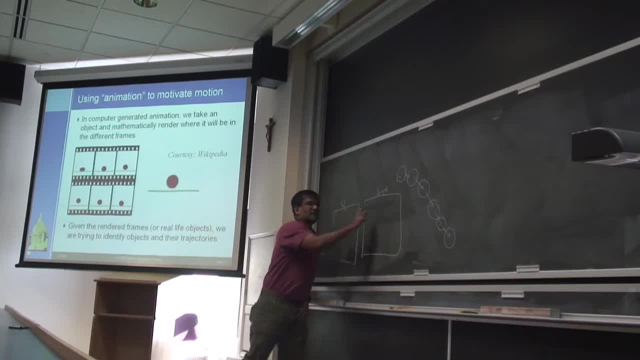 this stuff right, and I can search for whether this particular, this, whatever this rectangle was, happens to be anywhere on the screen. and the more I look, right, I can capture more than of the compression, more of the movements, but the computational effect goes way. 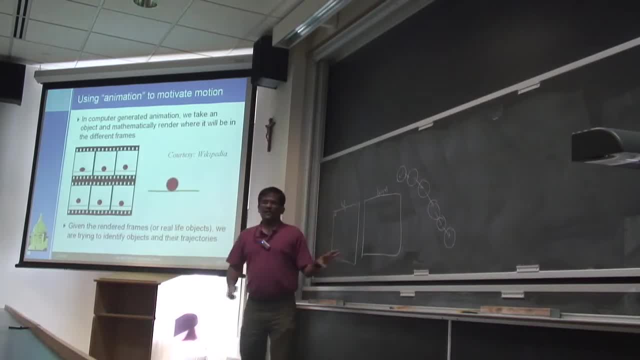 high right So I cannot afford to look through all of the stuff, so I'm restricting it to say I suspect that movements would have moved it from here to here. If I can't find it within that range then something is wrong, right. 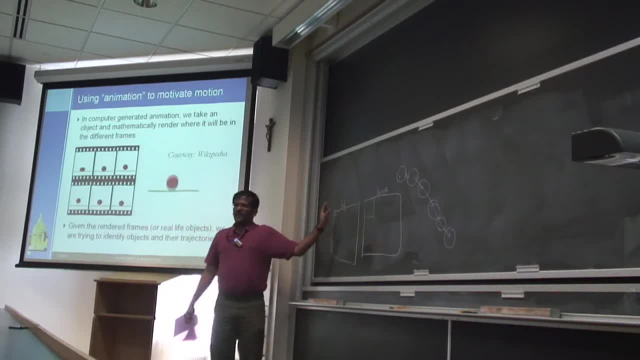 Otherwise I'm going to do this stuff. So I'm going to take each one of these squares and I'm going to see where it might have moved right. So the processing gets higher and higher, because this is, if I take 90-20 by: 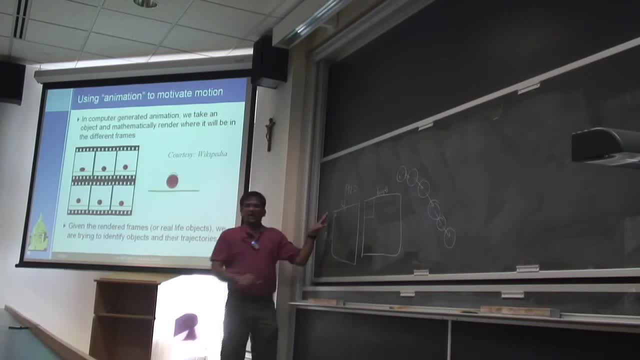 1080. so I have a certain number of blocks here and I have to see for each block I have to look in this bigger range, right? And I have to do it 30 frames per second, so the amount of computation goes way high, right? But 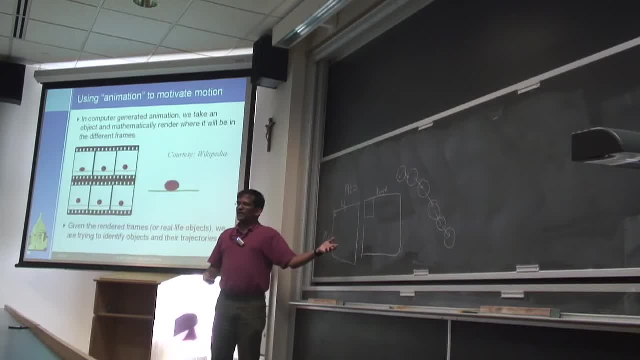 I have to try to do that because if I can find it then it's very good. It shows some illustrations of how it can help right, But the sky is the limit in terms of how complex you want to be right If you have. 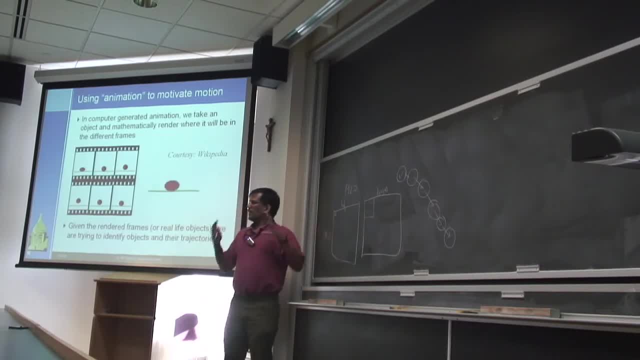 all the time in the world you may analyze this frame and this frame and figure out what has to happen and you go from there right And we'll see more complex, like in MPEG-4, and all those things are more complex in terms of what. 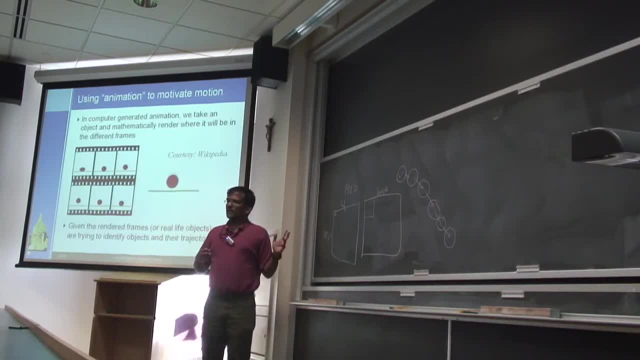 they look for not just blocks but objects and stuff. but essentially that's the idea, right? And how many of you like started doing the projects? in terms of like time to compress and all those things right, You may notice that it's extremely slow. 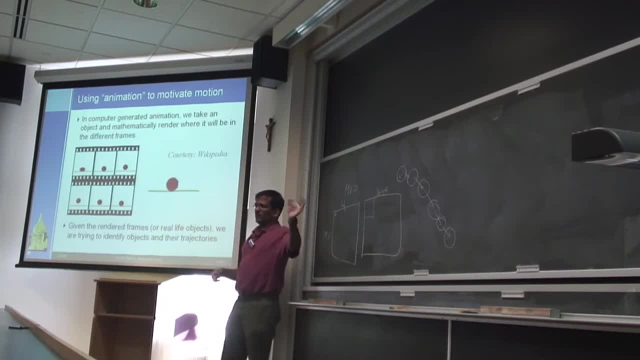 right. So, for example, this lecture I moved from my MacBook to a MacBook for transcoding right. So 15 minute lecture I started on Monday afternoon like 4 o'clock right. I had to stop it right now because it still needed 4435. 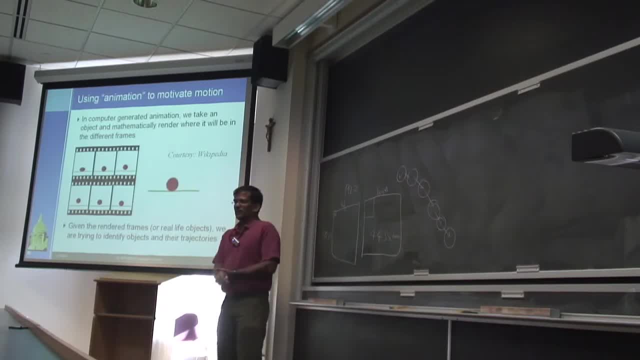 more minutes right To transcode it using so on my laptop. it takes like 15 hours, right. So I figured this is like the older machine probably take like 30 hours or so, but I don't know what this I didn't. 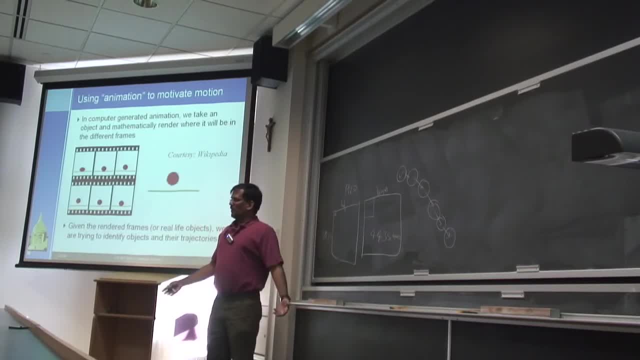 do the math to figure what how many hours it is, but I can't afford to let it go that long, right, It's been going on for almost like 40, 44 hours or so, right, And it's taking all that. 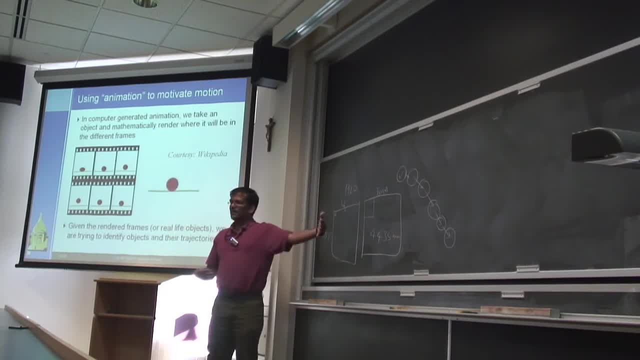 much time because it's essentially trying to figure out all this stuff right. This is kind of boring, not too complex, and if you see the equations and stuff, they're very simple. We're not trying to do anything pretty complex because even the simple stuff- the amount of data. 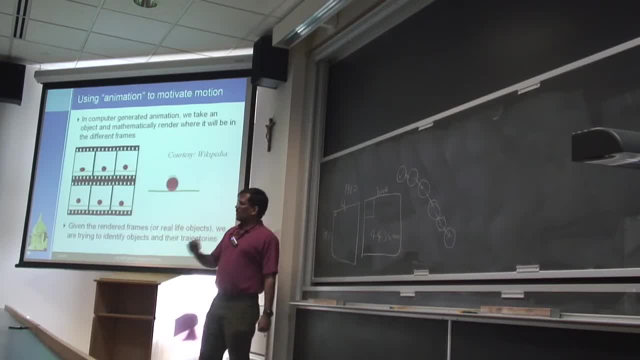 you're dealing with is massive right, And the good part of it is that it's not too complex. The good part is that all the time you spend doing this is worth it, because once you compress it, the decompressor is pretty trivial: All it has to do is 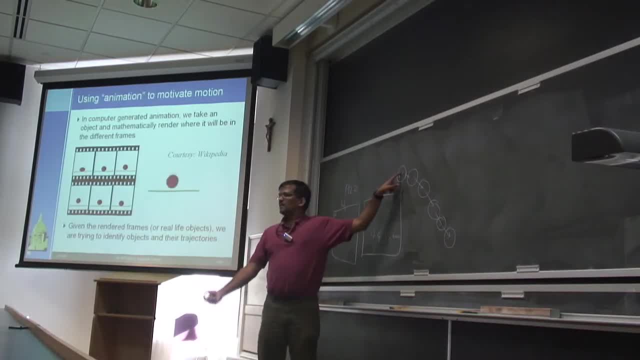 it gets this one and it gets something which says: okay, in the next frame, just take whatever the circle is and then plot it here. right? So I have to render a new one here and that's all I have to do. right? So you do all the processing on the. 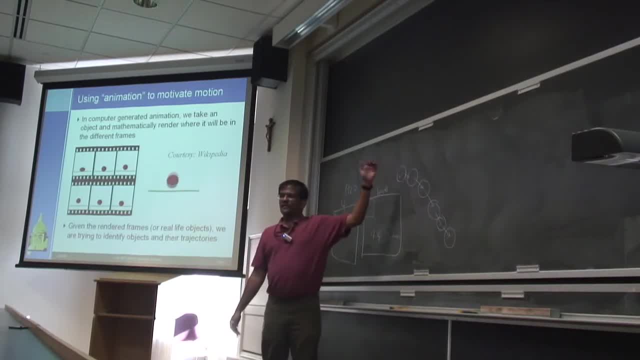 compression side. Decompression is simple because all it has is object and the motion. Does that make sense? So you're sort of trying to go back from these frames trying to figure out what really caused these things to happen. except you don't even know what the objects are. and 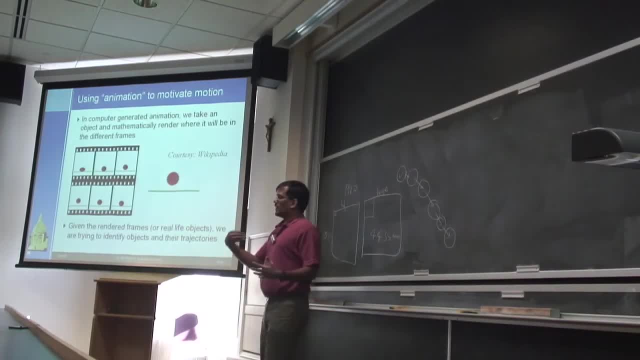 to make life interesting. it may happen that the two frames may not be related. In this case it's highly unlikely that suddenly something is going to change. but if you're watching a TV or something you may see, you're watching a game, you may see a certain angle. 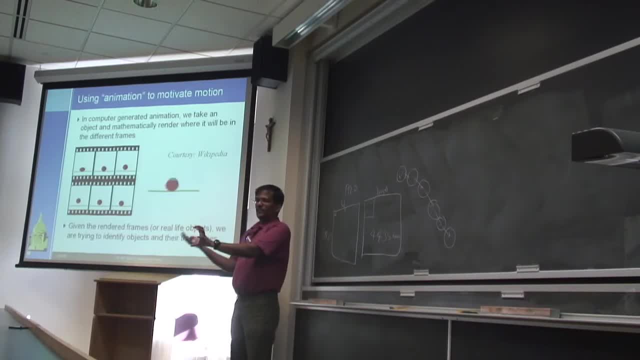 and you may see that future frames are all predicting from the previous one, like if you're watching a football or something, the next particular scene may be from a completely different angle, right? So these two may not be related at all. then you end up. 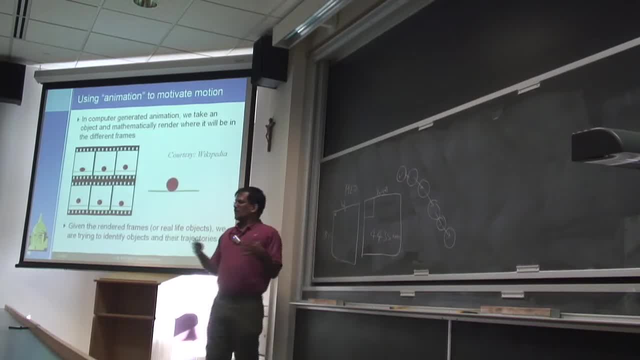 trying to figure out the similarity and at some point you realize that these two are completely dissimilar. so you have to go back right. So you also have to keep that in mind. You want to keep trying to find out what happened, but you can't afford to do it forever. 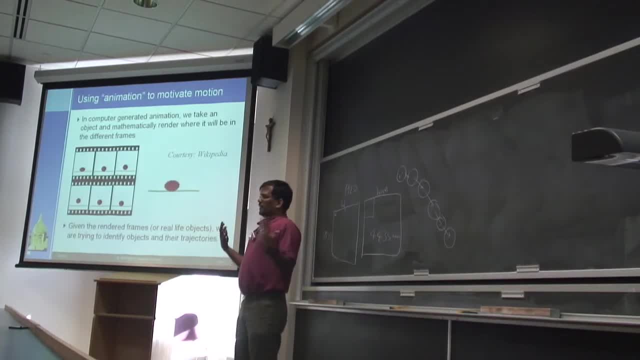 because it may happen that these two are completely unrelated, right? Either because they are completely unrelated or they're slightly enough unrelated that you can't really tell right. So think of your again a football game or something, right, So it might have more. 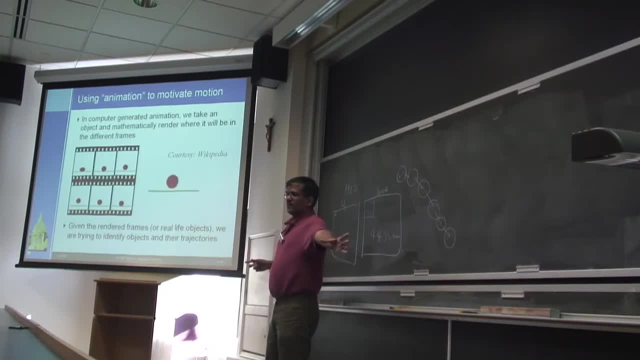 camera angle from, say, from here to this part of the state, if you think of this as the field. So it may still look like it's all green, it may still look like there's, you know, grass and all those things, but it's a completely different part. 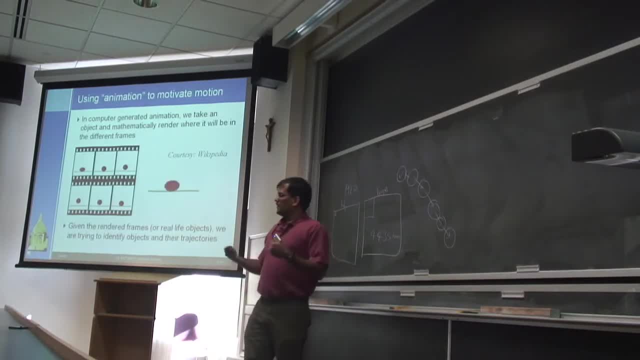 of the thing. so things change enough that you can't use simple tricks to get around from this right. So you need lots of processing. So that's the deal right. And to make so all the standards we're talking about, only tell you. 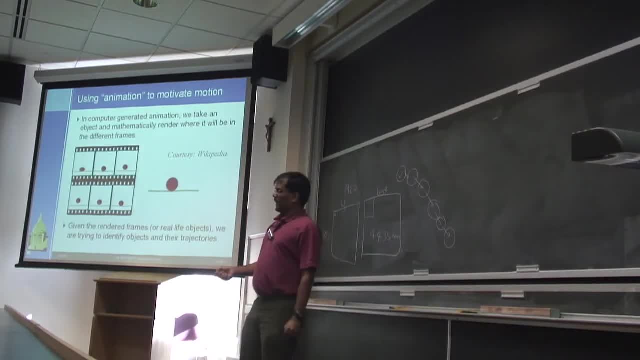 all these processes. They don't say what they have to do, right, So you can build a compressor which doesn't do any of this motion detection stuff. It'll be awful, but it'll still be whatever compression you're talking about- MPEG-4 or MPEG-2 or whatever. 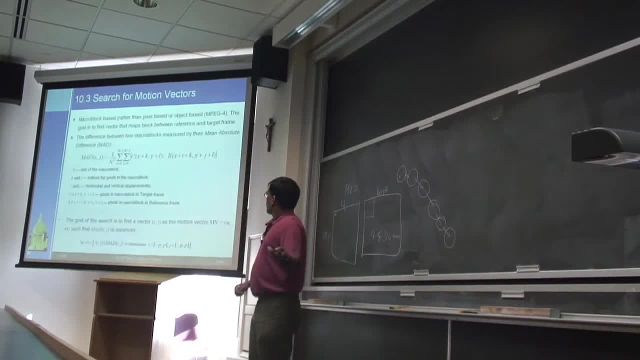 It'll be awful, but it'll still be MPEG-2 compliant, right? That's to make sure that you don't say what exactly has to happen. So you take a certain scene, you can use different compressors and you get different objects, different compression. 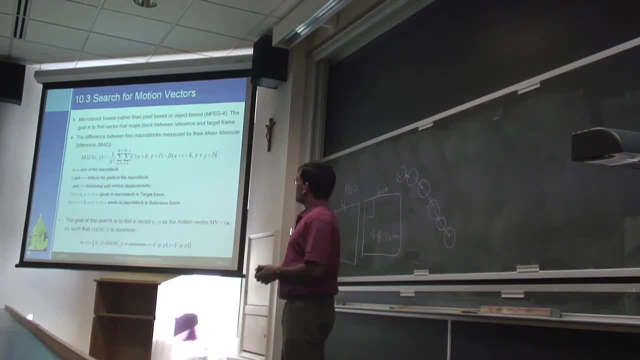 different. what have you? but they all look the same because they have to decode the same right. So that's the problem. So we're trying to figure out. so, as a first cut, we're trying to look at it as block-based, because finding out 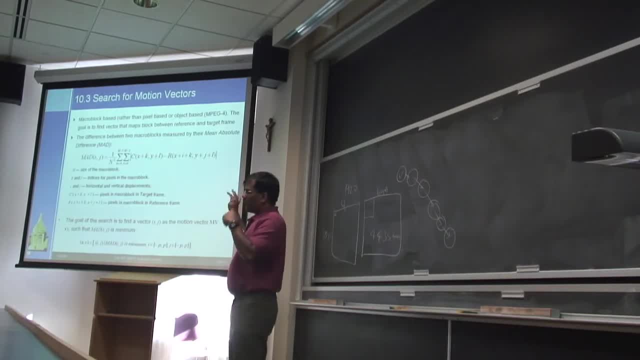 objects and stuff is way more complicated, especially in the earliest form of this technology. So you're trying to look at some block and you're trying to see where this block might have gone right. So the goal is to say: I take this block, let's assume 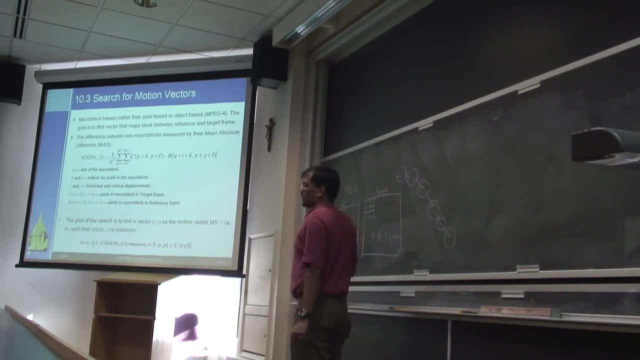 I have to look into this big area, right. So I want to figure out. I want to place this block over here, right, And do some sort of measure to see how similar the contents underneath it and this one are right. 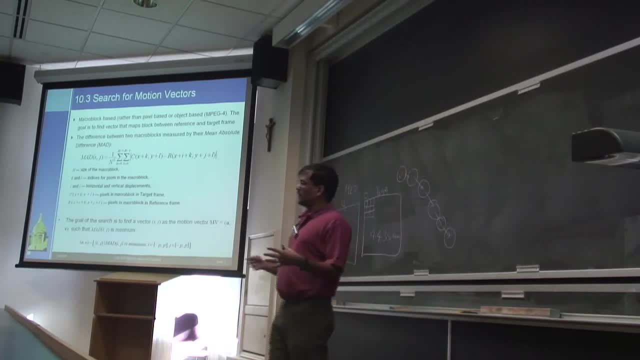 Some sort of a metric, And one of the metrics is the mean absolute difference, which tells you which compares these two blocks to figure out what's the difference. And there are other ones described in the book, right? So you want to find something. 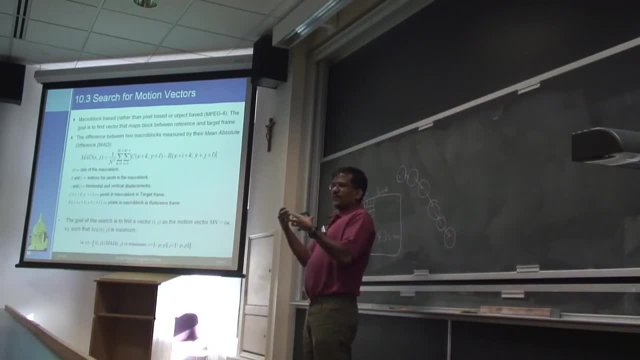 which can compare these blocks And hopefully they'll give you a number which says something about how good they are. So you figure out what this value is. Then let's say, you shifted one pixel this way. You do this measure, You move it one. 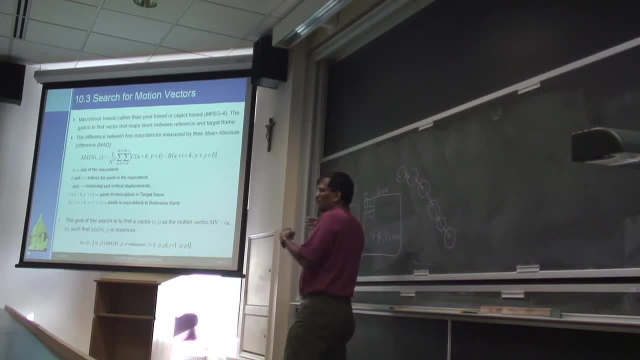 way do this measure You pixel. one way do this measure right? So you don't want this metric to be pretty complex, because for each of those iterations you have to take this block, whatever the block size is, and you have to. 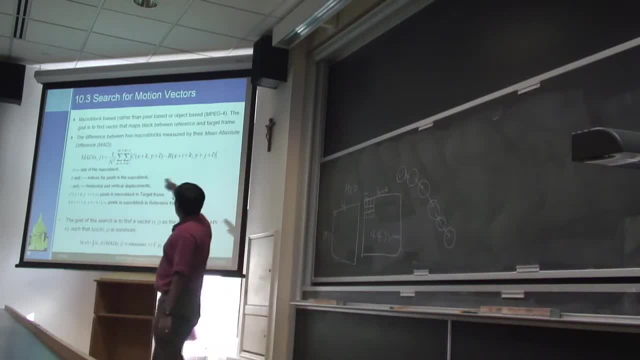 do this comparison And if you look at this, the equation for the mat, right, You're doing a bunch of subtractions and additions, right, But if you take an 8 by 8 block, so you're doing that many. 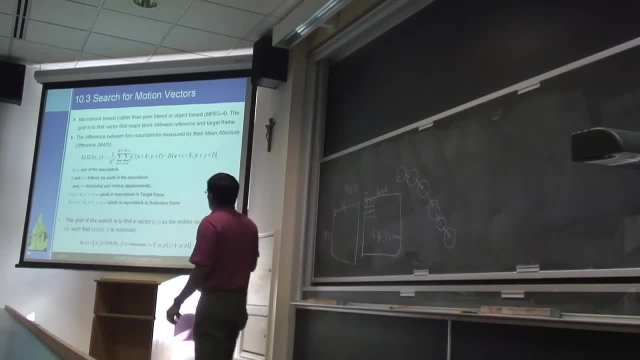 operations per block right. So that's the thing. So essentially, what you're trying to do is you do this stuff to other things and then find out the one to the least amount of differences And then you kind of say: if that happens to be here, 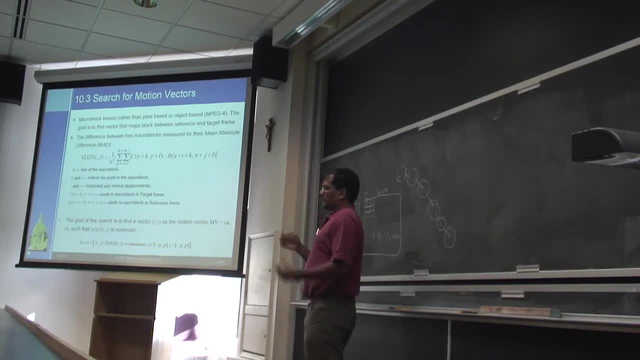 then you assume that this particular block moved over from here to here Because that's the lowest amount of stuff. So you're trying to generate motion vector from something from here to here, right? So there's something magical about mat, So you don't have to remember what mat. 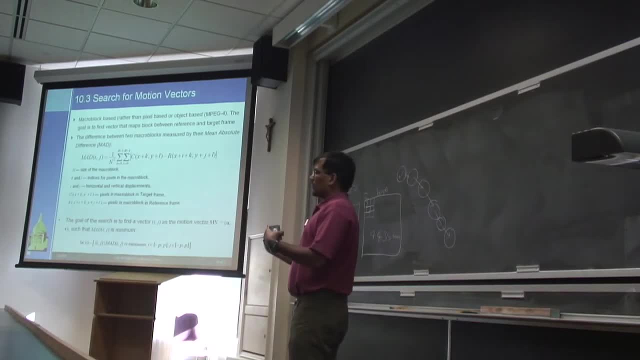 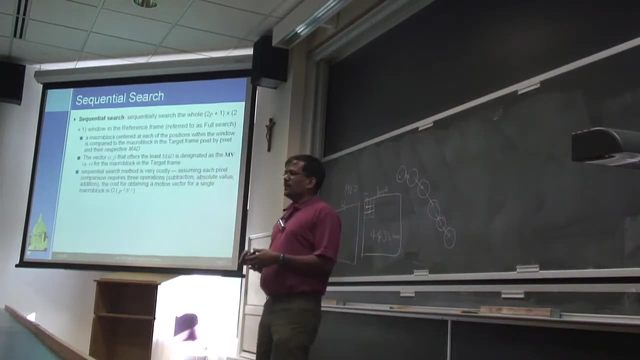 is, but you need some kind of metric which lets you compare two matrices and see how close they are right, And that's the goal. It gives you a number that you can use to compare two of these things. So there are a number of different ways. 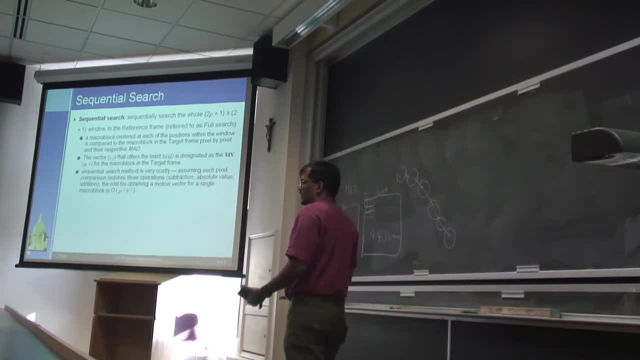 of searching this stuff And again, it depends on your encoder to choose the right one. right Sequential is whatever I was kind of explaining here where you take this, the P region, the region which you want to compare and look at every pixel, right. So you 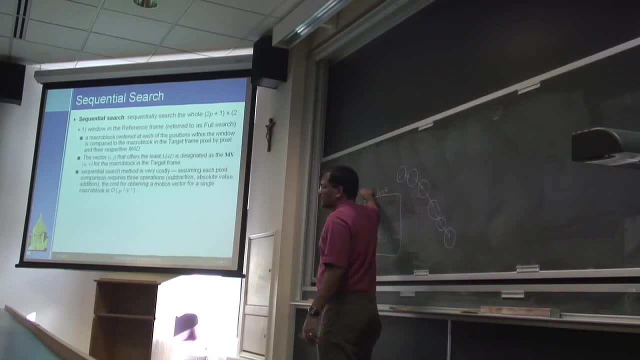 started, starting from pixel 0, pixel 1, pixel 2, pixel 3, and so on, And then you move one row down, two row down, three row down, all the way across, right? So this way you'll find. 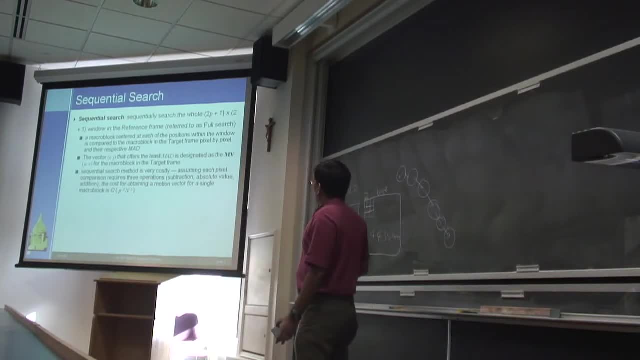 the minimum of this whole set right And it's also the most computation intensive right. So if you think of the subtraction, absolute value and addition, the book goes a little bit more detail. But essentially the complexity is O of P squared. 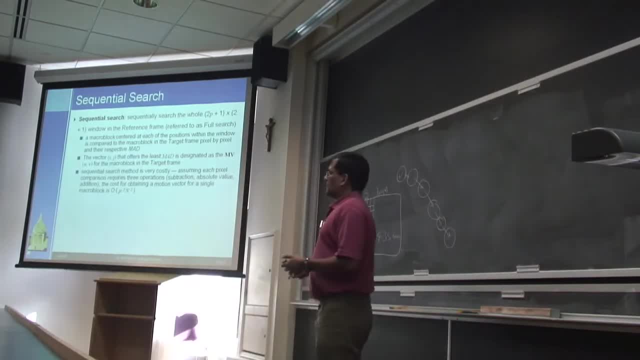 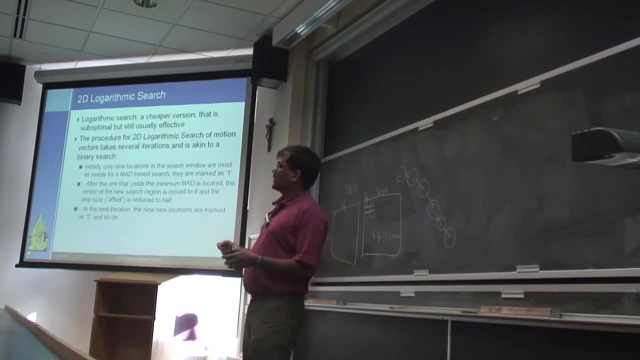 N squared, And so that's pretty expensive. So you're essentially doing it for every pixel, right? So there are other optimizations you can do. One is the logarithmic search, which is sort of like a binary search, right? So rather, 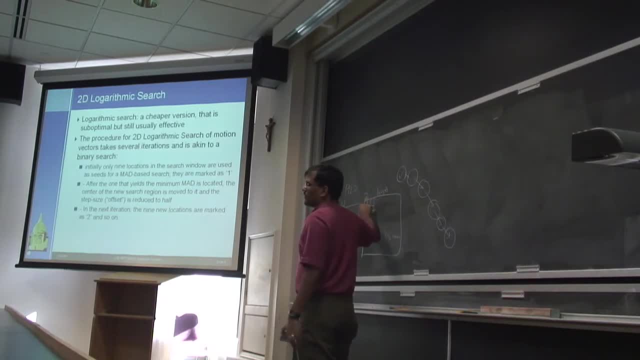 than doing everywhere. you kind of choose some points and you try to see which one seems closer and then use that as a neighborhood and then go from there right. It's very similar to the binary search, except it's in 2D, So 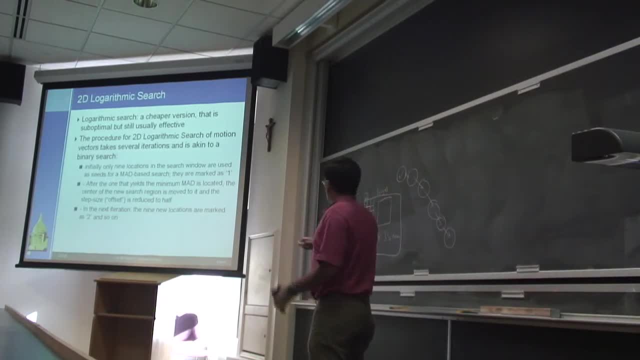 you assume that if you take this area and you are trying to match something of this spot, you assume that, let's say you chose these four areas right And you do the math at those regions. If the math at this region appears to be the smallest, then you. 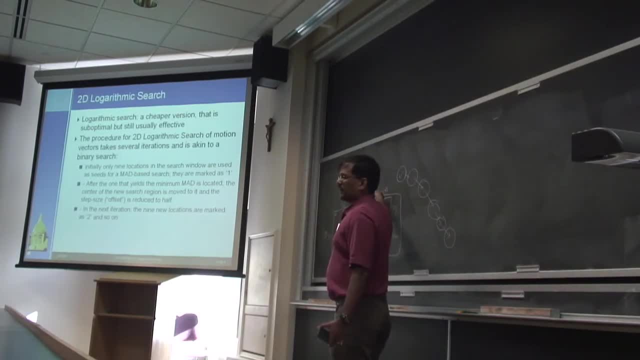 assume that the correct answer is somewhere along this area. right, It may or may not be true, but in general you assume it's true. So then you start going from somewhere here and then you do the same thing: You split this area. 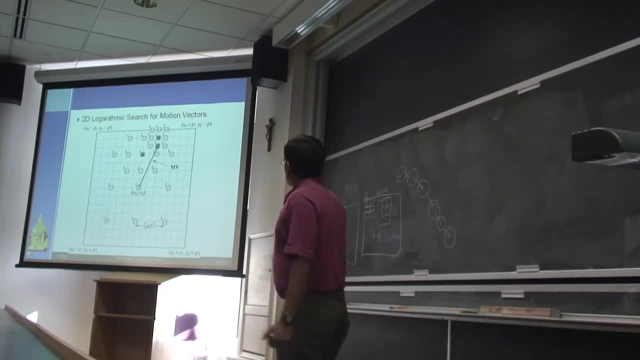 into four, and then you try to find out where they are. So the book has illustrations, So essentially you take this. the one is the first round of the object. So rather than going through every one of these pixels, you choose those one points. 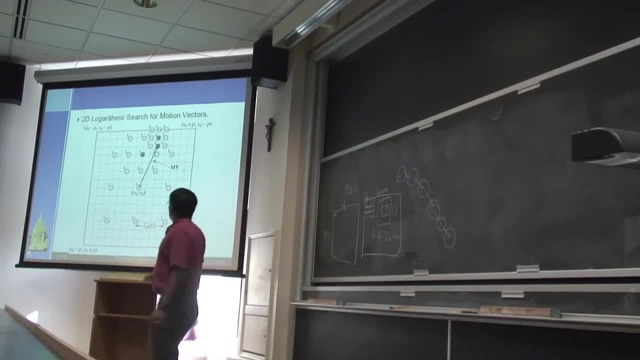 and find out where the minimum is. It turns out to be that point right, That darkened one. Then the next iteration: you choose a smaller rectangle around that one right, And you try to find where it is, And so on and so forth. 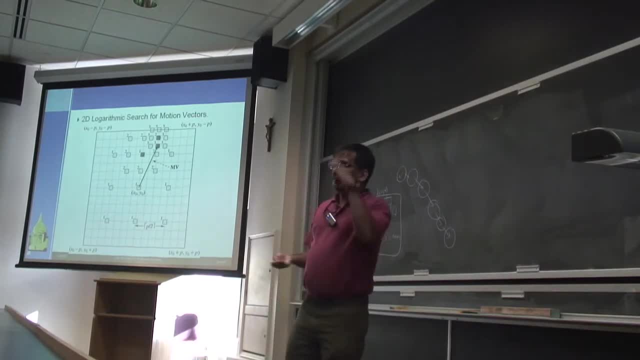 And essentially you find this stuff. So it goes as a kind of binary, kind of search And again. so if you take an algorithm course, you probably can come up with much more complex, much more realistic algorithms for doing this. But the reality is, 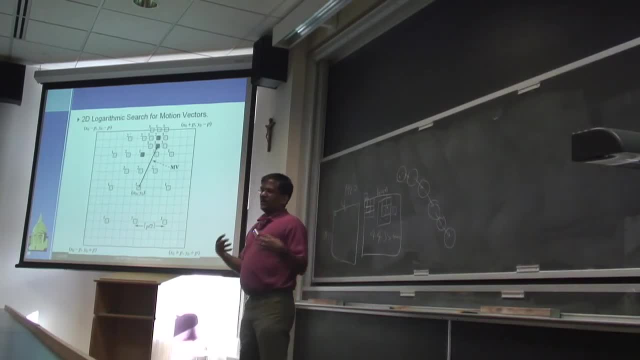 you have to do lots and lots of this stuff, right? So the code size and the time to do it is a lot more important than anything. right, Because you have to for every frame. you have to do this for every other frame And, as you will see, 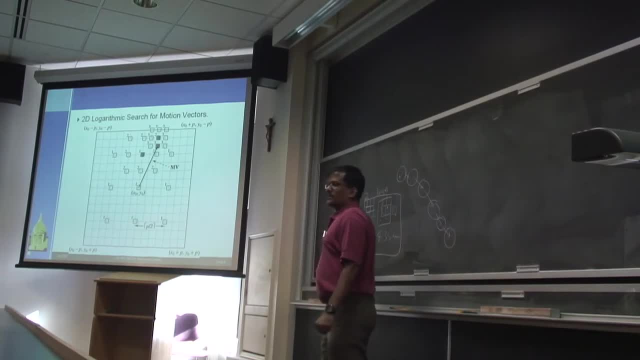 the complexity is, you may not be able to do, you may not have to do it just with the past frame. Good compression would actually go like certain number of frames forward and backwards. right, And that's what MPEG and all MPEG 2. 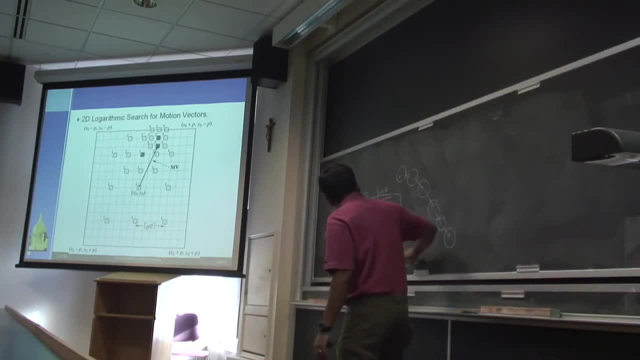 and 4 and all will do, which is essentially if you have a set of frames. in the simple case we can look at the previous one to figure out what the next one is. that's the forward predictor. But in more realistic cases, if you can analyze, 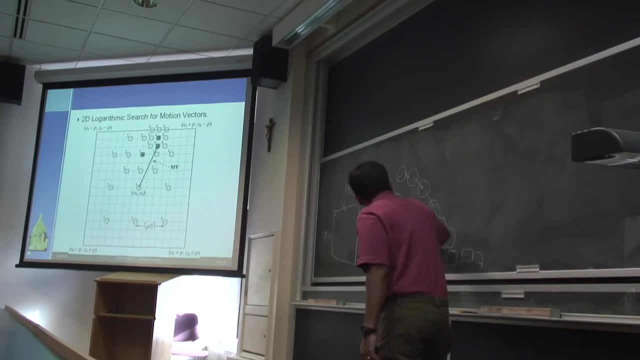 a whole bunch of these frames. you may find out that this frame and this frame are related to this and this frame, right? And this is related to something over here and this is related to here, or something like that, right? So think of. 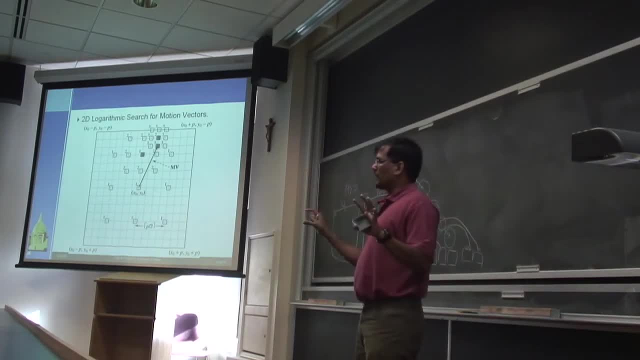 if you think of a movie and stuff, you know you have two cameras going back and forth, So you want the prediction to go further as far as possible. You don't want to go to infinity, but you maybe have to go through this a lot, right? 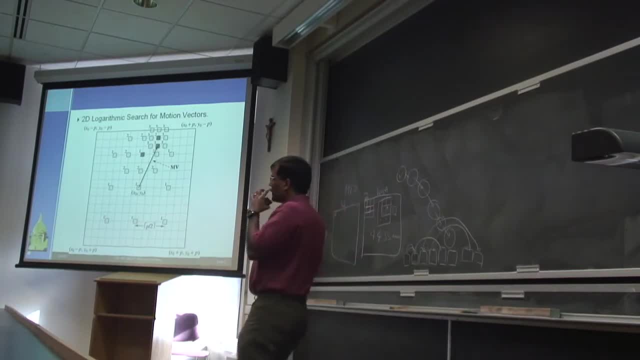 Because that's what happens in real life. you know you have these different scenes kind of glued together So you want to do as many competitions as possible. Each one of these frames is big as 90-20 by 1080, kind of thing. 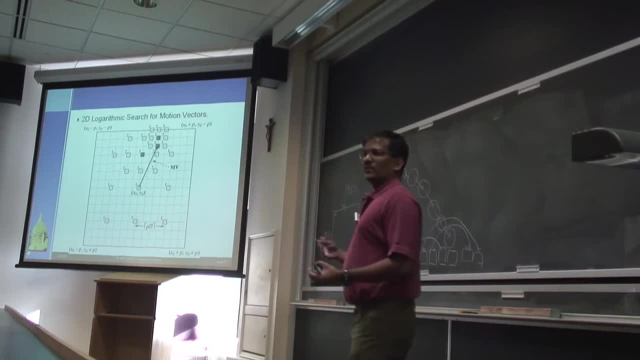 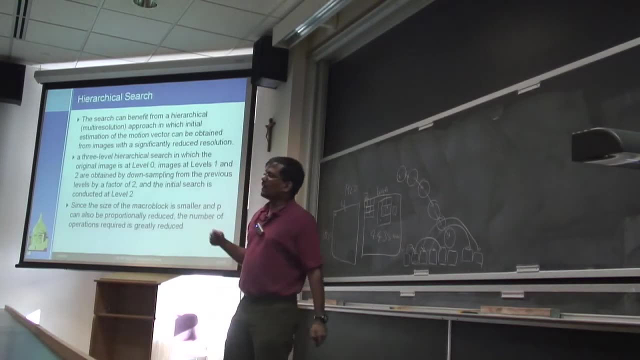 So you want to be able to do this lots and lots. So that's the challenge you're trying to do right, And the last approach that the book describes is the hierarchical approach, which is sort of like again like your binary search. 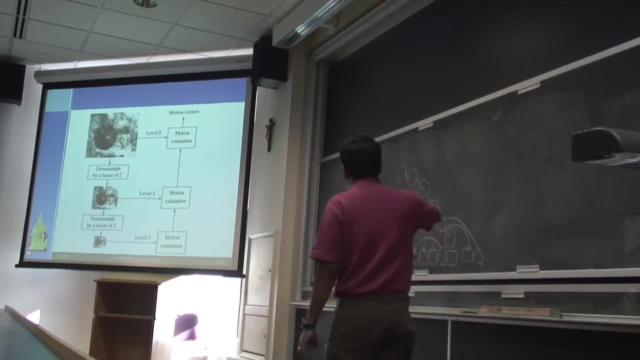 Essentially what you do is you downsample the image, right? The idea here is you take this big image which is over there and you're trying to match something. So, let's say, you downsample it by 2,, which is you divide. 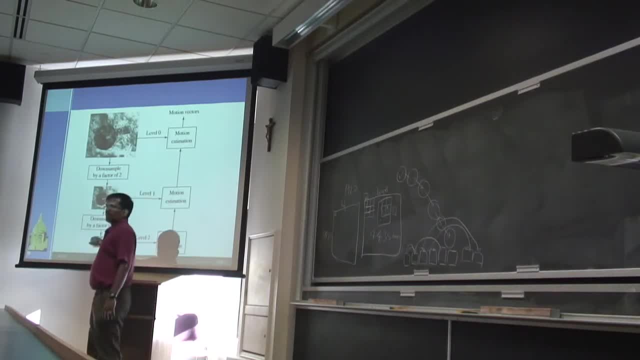 all sides by 2. So you have a far smaller image, right? Then you try to find out, and of course you have to downsample your block too. Then you try to see where that block matches here, right? So if you do a double, downsample it. 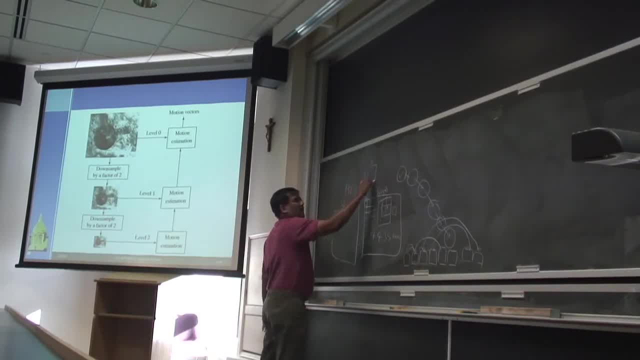 twice and if you have a 8 by 8 matrix that you're trying to do right. So essentially you can do a 2 by 2 matrix, that you change the reference one to a 2 by 2 matrix and 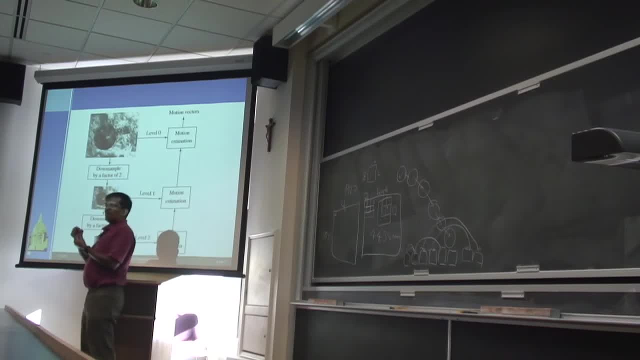 you made your whole image to be small. Then your number of competitions becomes smaller because you're trying to match on this one. So again, whichever region you see a match, then you go back to a higher level and then start from there to. 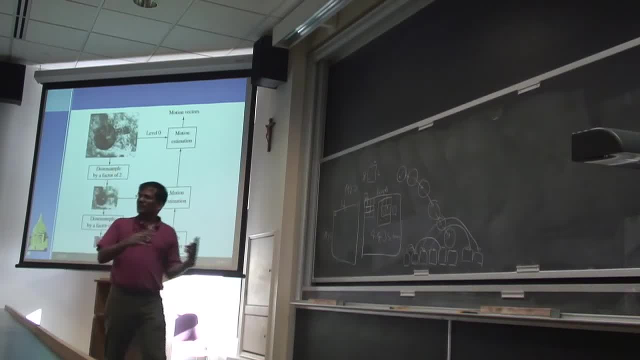 look around and then go back right. So it's sort of the same as what you did with the logarithmic stuff, except you do this downsampling and you're searching. So the idea here is if it tends to match at some point here. 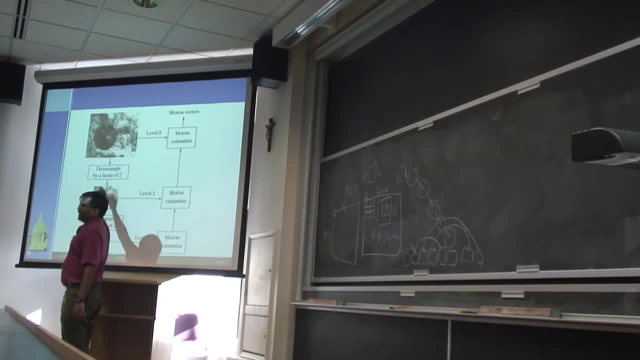 that will map into a 4 by 4 region over here, right, And then it gets mapped to a higher and higher region. So hopefully that will help me find these things faster. right, And again, you can think of other ways to do this. 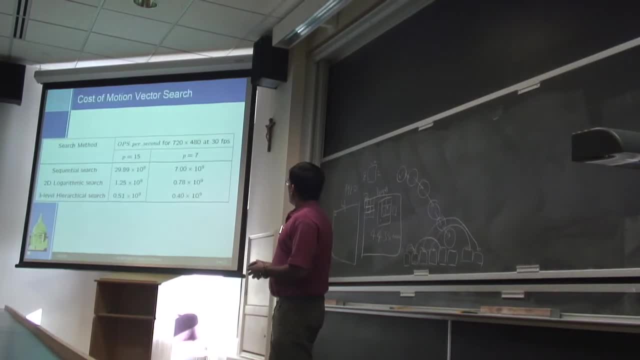 stuff and the key here is these things should be fast. So the number of operations per second for a sum of 20 by 480, which is the DVD size, 30 frames per second. So if you have the p equals 15 or. 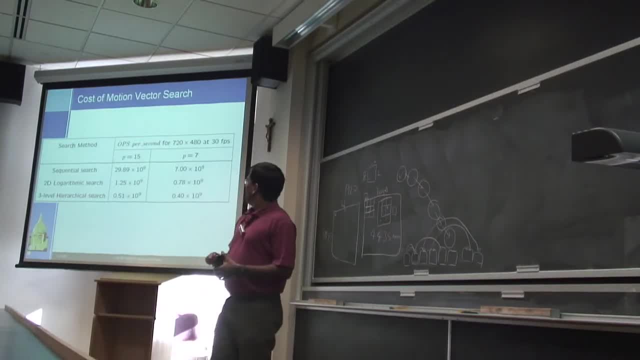 7, it tells you how many operations it has to do. right So the sequential search. so if you ignore the billion part, right So the sequential search, you have to do 29.89, but with a 3D hierarchical you bring it. 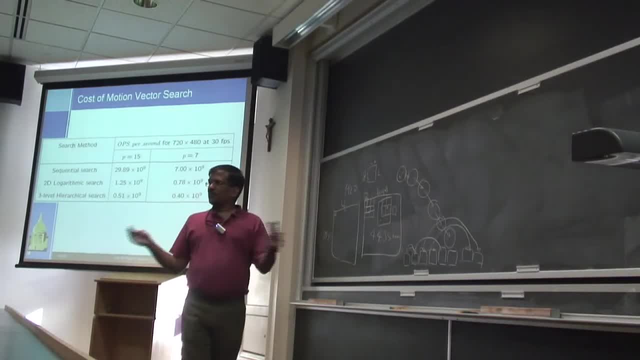 down to 0.51, right, So it makes a big difference in terms of how well, how much competition you have to do. but again, the catch is there may be cases where these things miss those stuff If the movement is subtle enough. 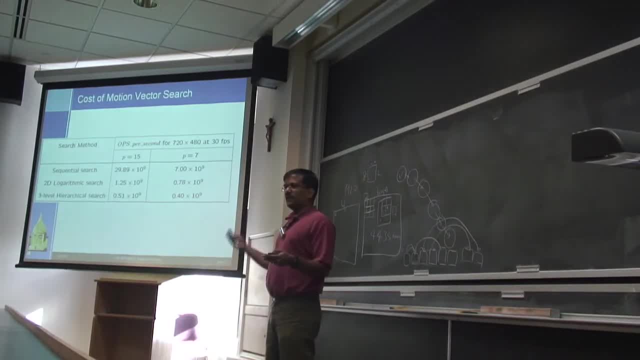 you might be able to see what happened right. And again, if you come with newer codecs, you're free to do whatever you want. You're free to do, however. you find this stuff. All you have to find is which block moved from one to the other. 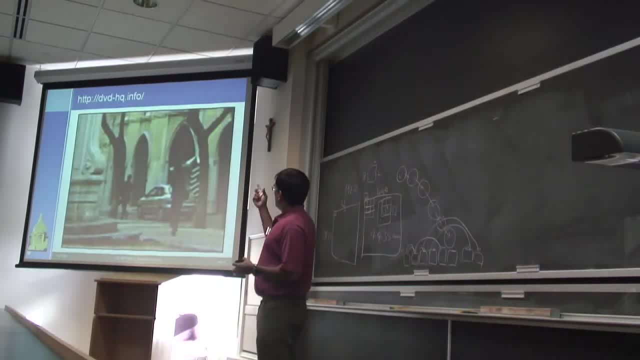 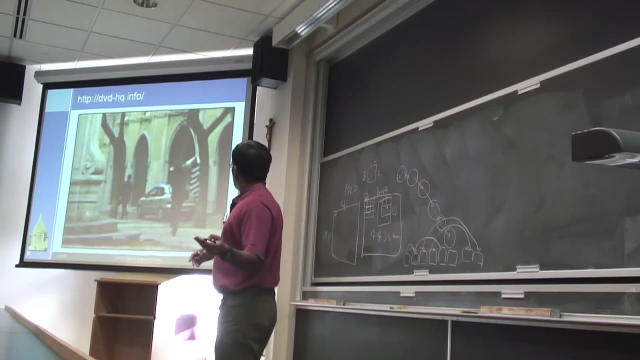 to encode, right. So again I found some image on the web to see how these things kind of pan out, right. So dvdhqinfo had this one super grainy picture right. So essentially, if I go back and forth, right. 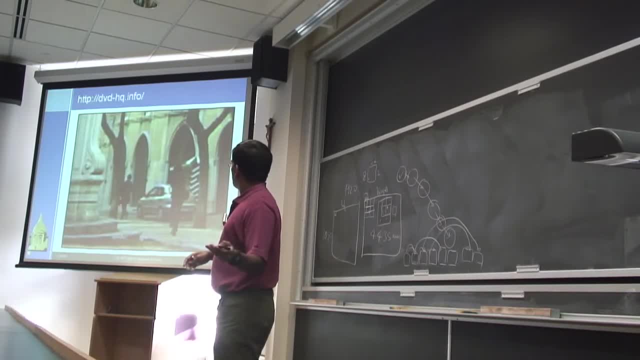 You see that between these two frames, right, I'm going back and forth. right, The car kind of moved, people kind of walked, people kind of moved a certain way. right, The buildings hopefully didn't move because the camera was not panning right. 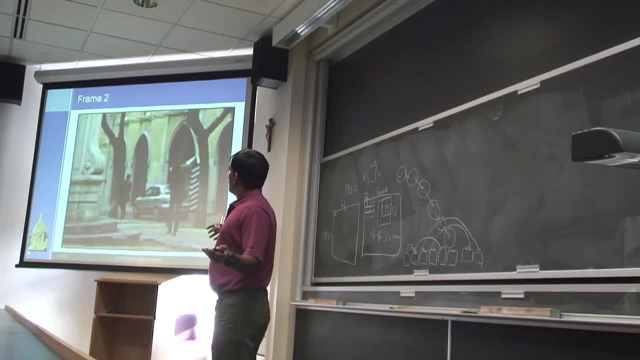 The camera was looking from one angle. So what you're trying to do is you have JPEG artifacts and stuff on the thing. So if you look at the column right, If you look at the pillar on the over here right, The pillar did not move. but you see, 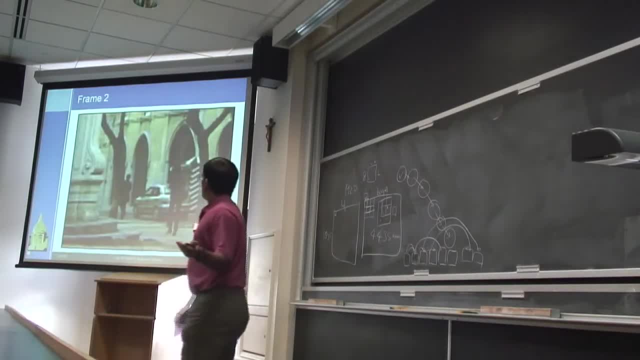 the JPEG artifact, making it look like it's kind of moving, because the picture looks different, right? So hopefully, if you can figure those out right, All you have to do is I would have to encode something about this person, something about this car, something about. 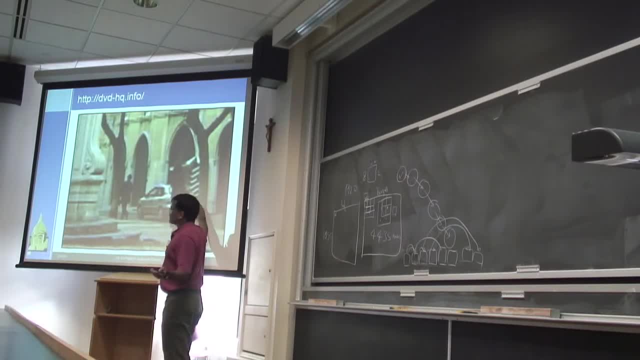 this person and something about areas that this car, once it moved, would be visible now, And something about areas that used to be visible- not visible anymore because the car moved right. So that's what I'm trying to find out. So, if I can find that all, 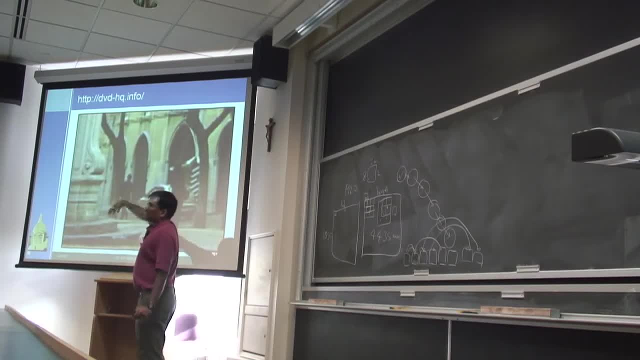 I have to encode is sort of the action happening around here. The rest of the scene, nothing is happening, so I don't have to subtract anything right? So again to show what the macro blocks, so essentially you know, for this particular 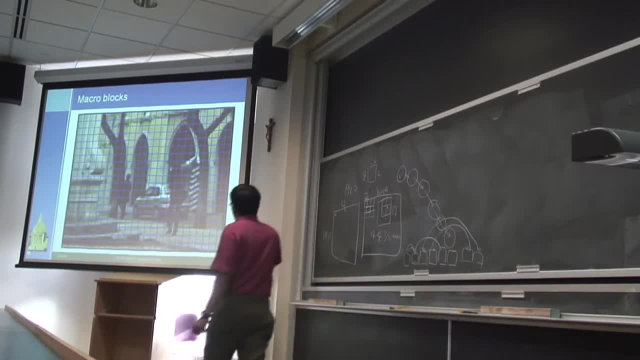 scene. there are that many macro blocks. You have to look at each one of them. So you look at this and you're trying to look at where the corresponding one on the next frame and trying to see where they matched right. 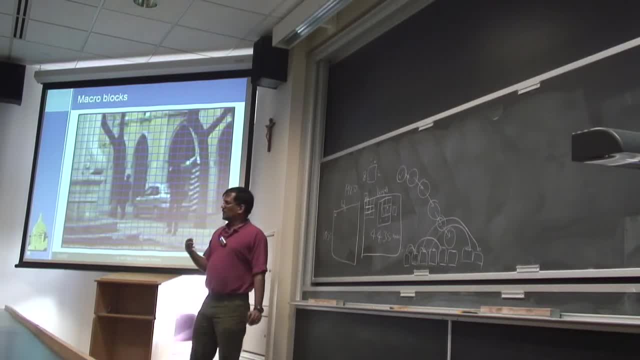 And if you look at it visually, there's not much detail. So you know, you may or may not be good all the time and that's why the difference in vector comes. So to explain this stuff, they took some blocks right, They took the 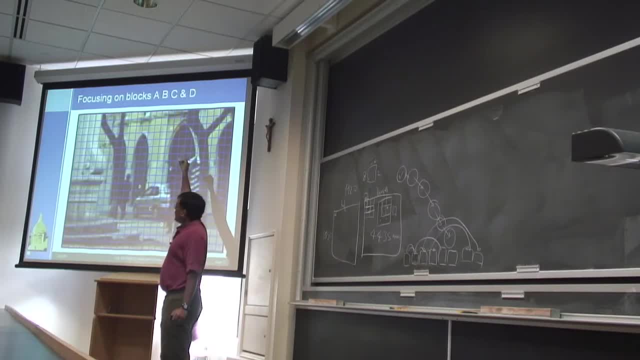 A block, Nothing should change because the building did not move. But you see, over here things change because there's part building and there's part car. right, You may be able to see the car. So when the car moves you see something changing, even though 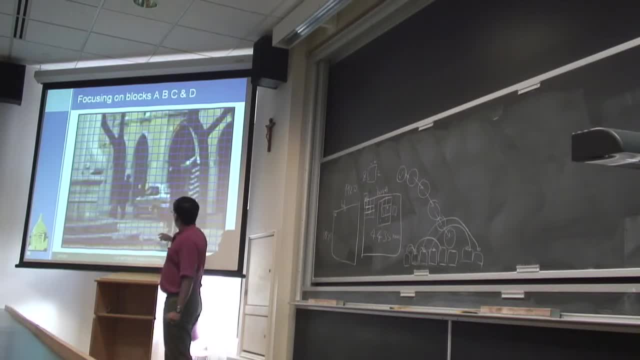 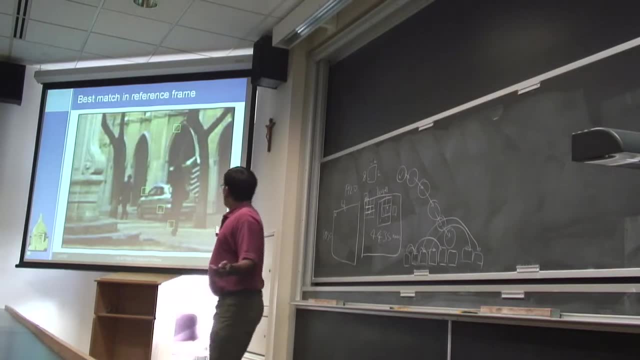 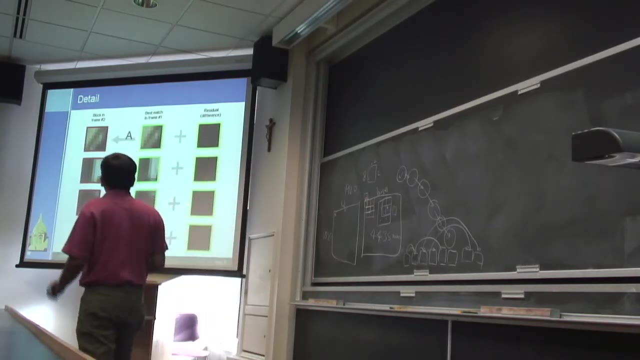 this line would be the same Over here, the tires have obviously moved and something. and this is the person, so their feet will move, So in the new screen they will change. So they go through the analysis and then they say what? 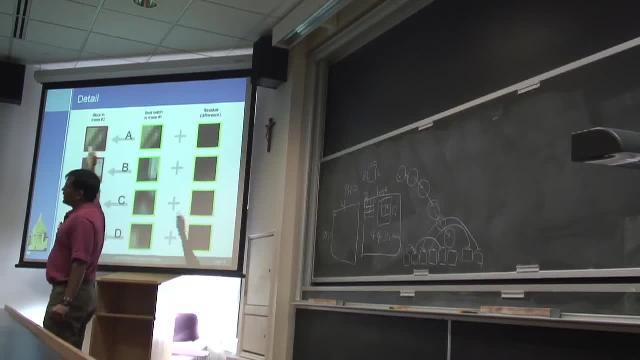 argument they use, But essentially they figured out for the different A, B and C. these are the best frames, right, And this is the residual. Obviously, we can't see this in the display here, So these are the difference between these two. 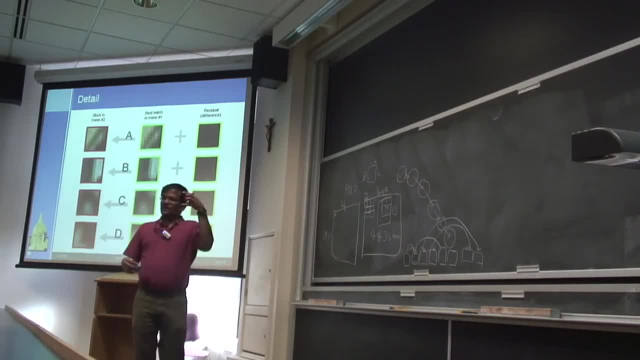 images right. So, which essentially means that you are predicting this block goes to another block, You have the vector for it And once you move it to the new location, you have to apply this difference because things change slightly And if you look at here, it looks like it's completely black. 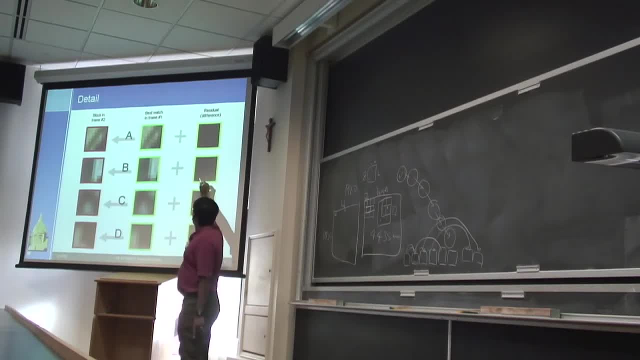 But if you look on the- maybe on the printer or on the PowerPoint, you may be able to see a subtle, slight color here. I don't know if you can see it in the back right. So there's some difference right, The key, that you cannot see. 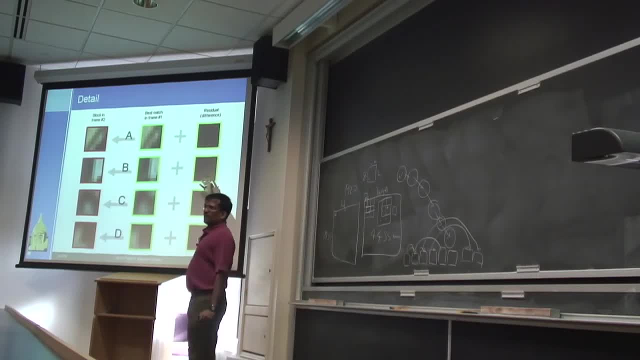 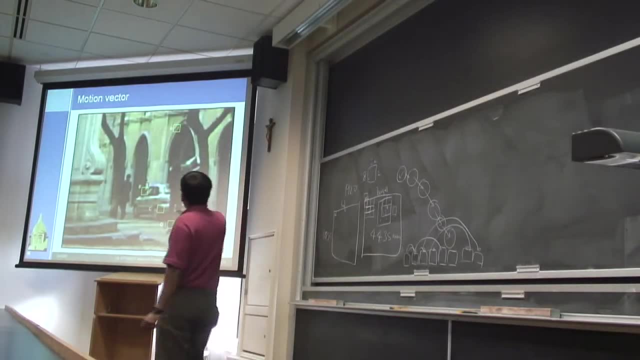 much is the key, because that means I can compress this very well, because it's mostly black right, So I can still make it look good. So in this sense, if you look at the, I forget which one is the new and which is the old right. 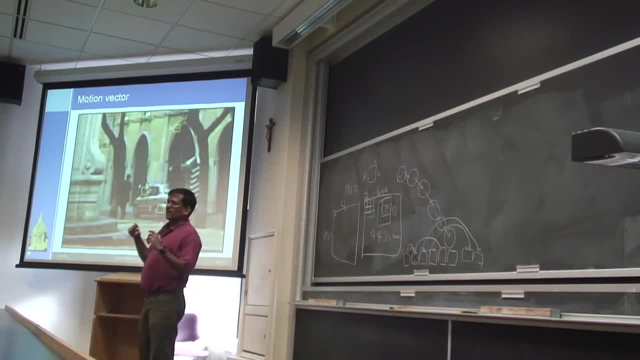 So essentially, for each of the blocks, the motion vector says where they are in the future, right. So A happens to be A didn't move because the building did not move, But the other ones, they you know. essentially, I think the green is the old one and the red 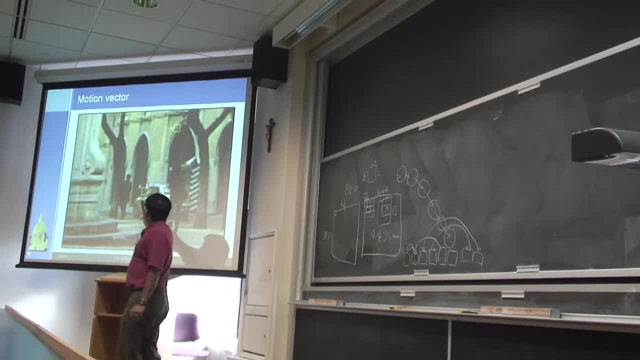 is the new one, right? So you say it moved from here to here. So you see the different blocks moved differently in different directions, right? So this one moved this way, this one moved this way, this one moved up there And 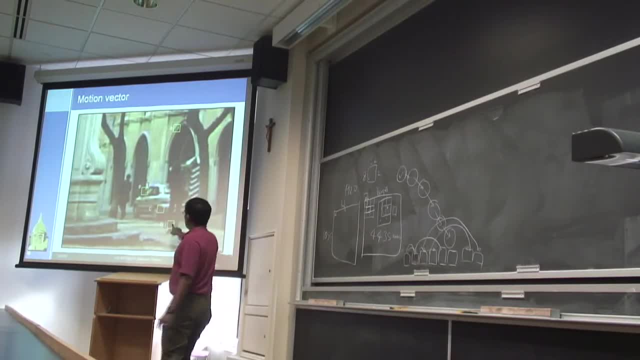 the motion vector, you're saying it's a new block, So you're going to say this block, motion vector- is a vector which is this much movement, this block, this much movement, this block, this much movement on the certain direction, and the difference between- if you 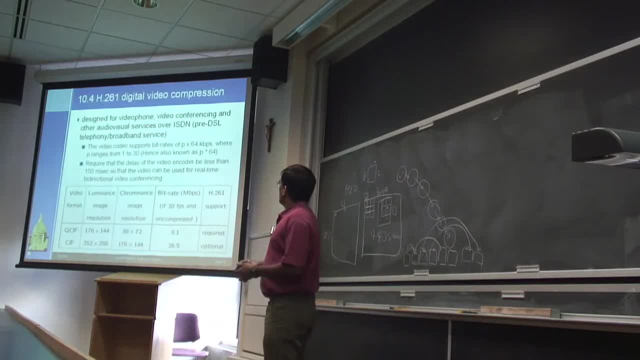 just move it and then that's what you're transmitting. Does that give a sense of what is being done? So that will give us enough background to start looking at how some of the media compression algorithms are designed. And again, as we move forward, as the standards move, 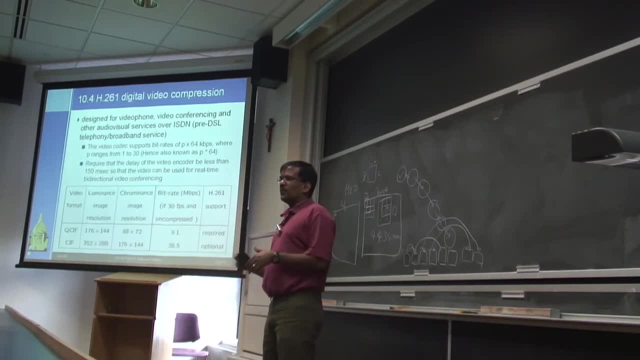 forward. you have more and more complex videos, So we are going to first look at H261, which is one of the compression algorithms. It's a standard, So H261, H264 is M.4, which is more of the modern compression algorithm. 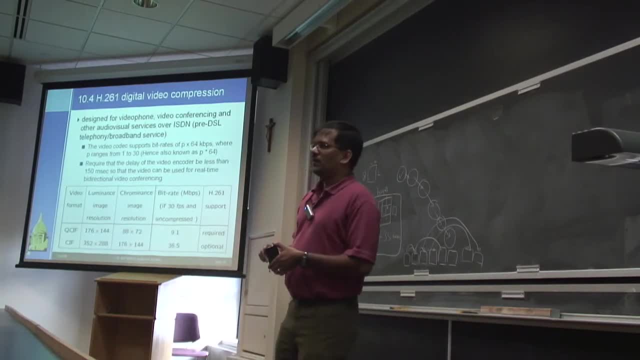 So this was designed for video conferencing over ISDN networks. Come here: if you've heard of ISDN network, I'm surprised, because telephone companies fought really, really, really, really hard to kill that technology right, Even though it's supposed. 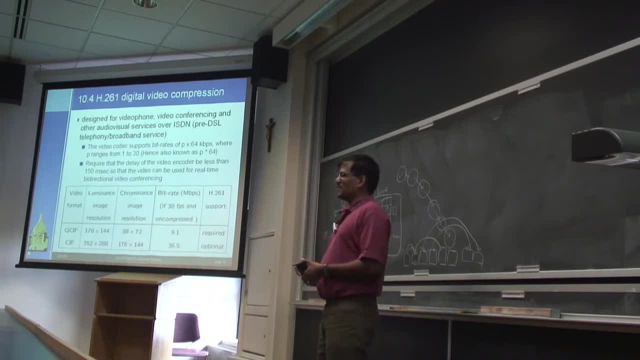 to be telephone technology. So where do you? did you use it for something? I'm just worried, I don't know anything about it. So ISDN was supposed to be the broadband before DSL and all came out right. So ISDN was supposed. 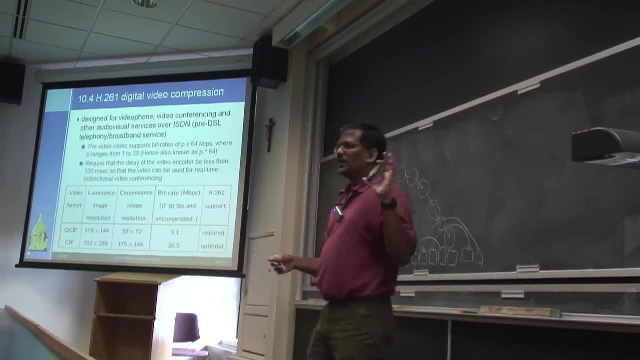 to be something that the telephone companies could sell- I think it came out about in the 80s and stuff. So you can sell. they were able to sell it at increments of 64 kbps, right, So you can get 64 kbps, which is sort of. 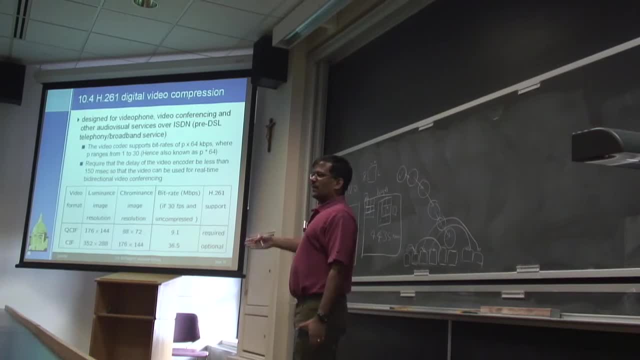 what you get for your, for a home phone, And you can get 128 and so on and so forth. I say that they were trying to kill it really, really hard, because when you, this is the days when there used to be dial-up right. People used to have dial-up which is 55 or so, which is sort of like a kbps. So if you wanted faster, you wanted like a 128, which is like two dial-up kind of thing. So the way the phone companies were charging was: the ISDN at that rate. I think when I checked in mid-90s it used to be like $300 or something right, Which clearly is kind of weird because you could get two homelands into your house and have two dial-up modems and pay like $20 or something for your dial-up, so you get like $40 or whatever, maybe $50, $60 or something, right? So they were selling it at this enormously pricey thing to get 128, kbps or what have you right? 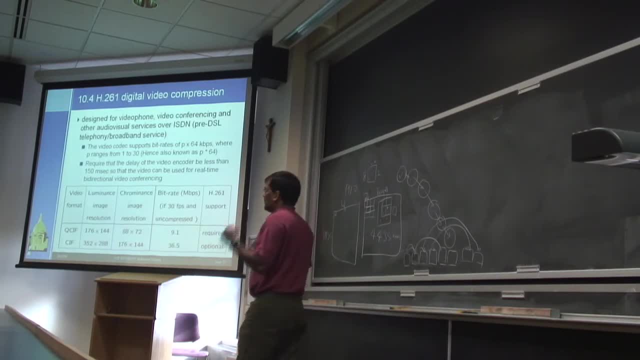 So they really, really tried super hard to kill the technology. They finally killed it. then they realized that DSL came, and you know the rest is history, right, So anyway. so one of the things that they wanted to do was be able to have video. 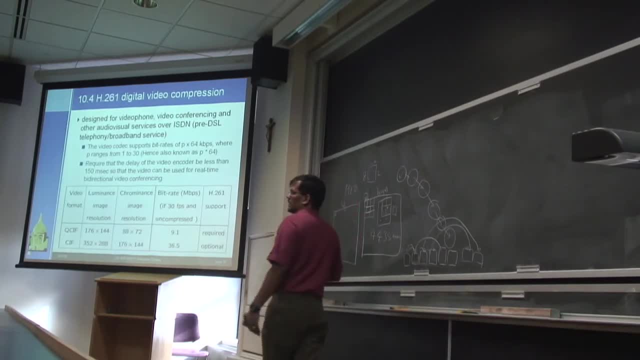 telephones. If you look at any of the advertisements from 80s and 90s- right, the future they imagined was people would remove their phones and then replace them with a video phone, right? So if you look at the AT&T ads from back then, people would: 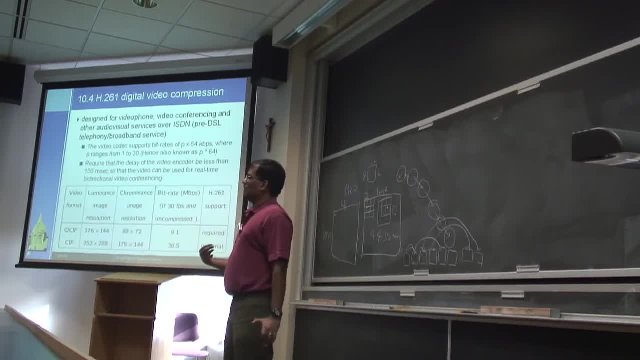 replace their. they imagined people would replace their phone with a video phone, So the technology was developed as a way for you to communicate over ISDN networks for video phones, right? So there are a lot of constraints that were put in place because it was designed to work over. 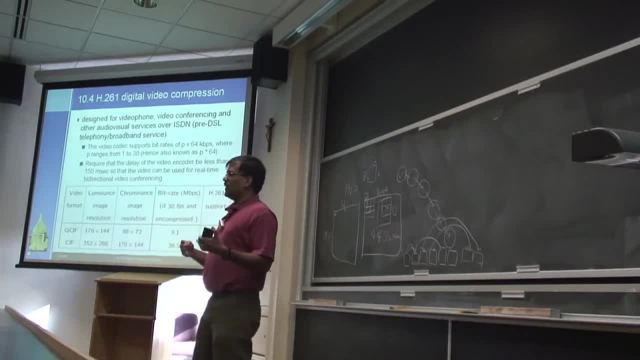 ISDN right And some of this, many of this stuff is no longer true because people are not kind of stuck with the ISDN technology. But a lot of the technology they use for the compression gets carried over because they turned out to be fairly good right. 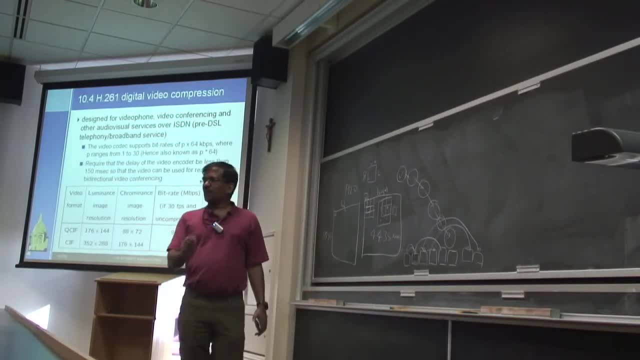 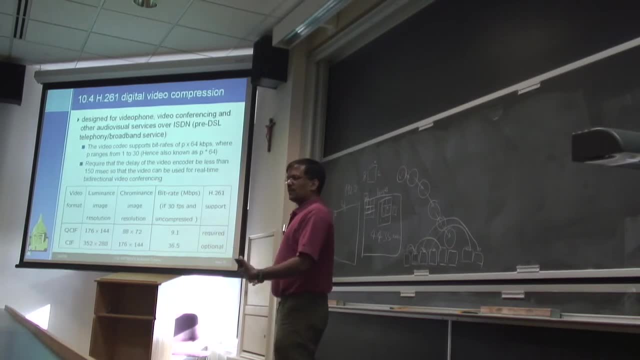 So one of the aspects they had was it has to be multiples of 64 kbps, Which means that the output has to be multiples of 64 kbps, because that's sort of how ISDN was sold to you. So you either get 64 or 128. 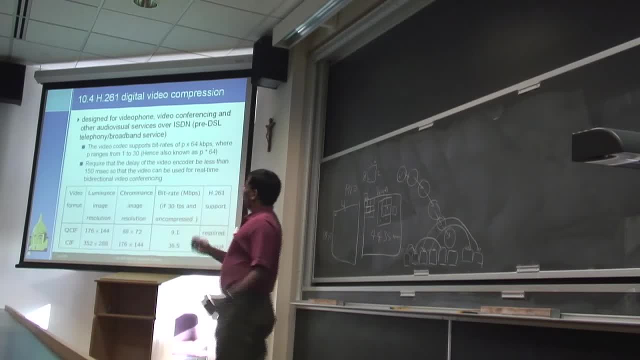 or whatever. So the compression has to be created in that ranges. And they also had a goal that the encoder has to be less than 150 milliseconds. Again, this is supposed to be a video video phone, So 150 milliseconds is deemed to be. 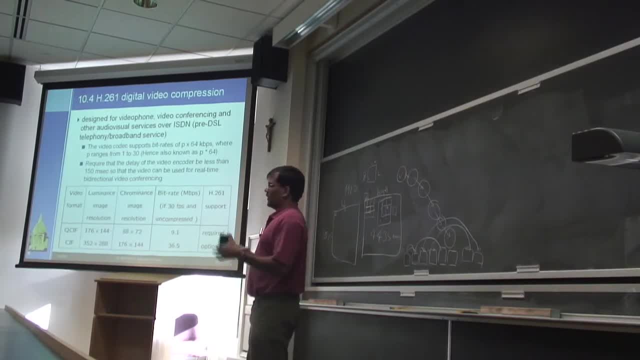 when you notice that things were off because you know the, it has to encode and transmit it over the wire so the other person can see it and all those things. So those were set right. So those two parameters were set. It has to be within. 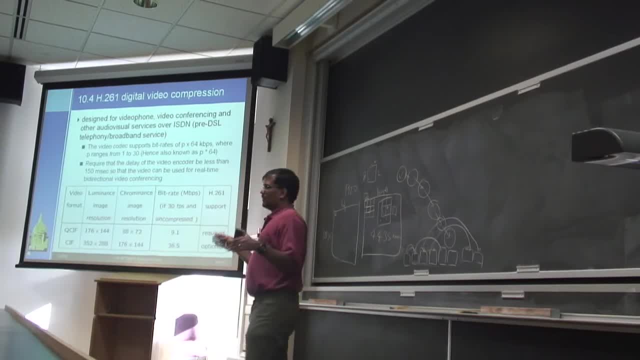 64 kbps, Up to 30 times 64, but essentially multiples of that. And the encoder has to happen within 150 milliseconds- And this was in late 80s and kind of stuff, So 150 milliseconds was a lot more bigger deal for encoding. 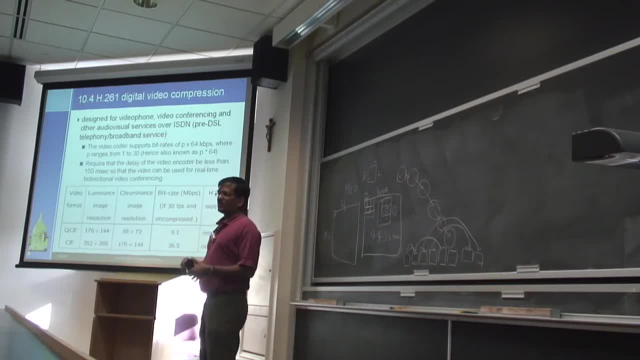 than it is for many of the modern stuff. right, So you can imagine your iPhones and earphones are probably way more powerful than the computing that were available back in the days. So they wanted to do SIF. Remember the SIF? we kind of 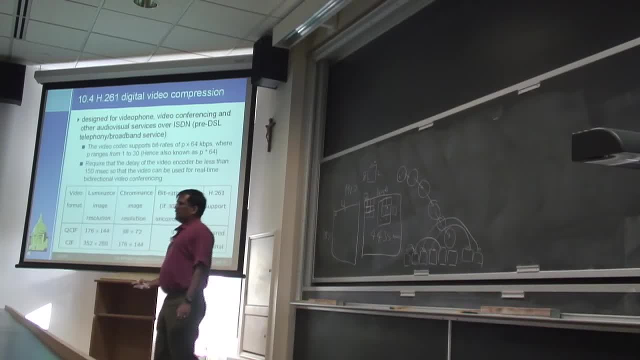 mentioned the image size. They wanted to do SIF but really they can only do QSIF, which is quarter of a SIF right, But the dimensions for the luminance and covalence are here. So essentially they are doing 4 is to. 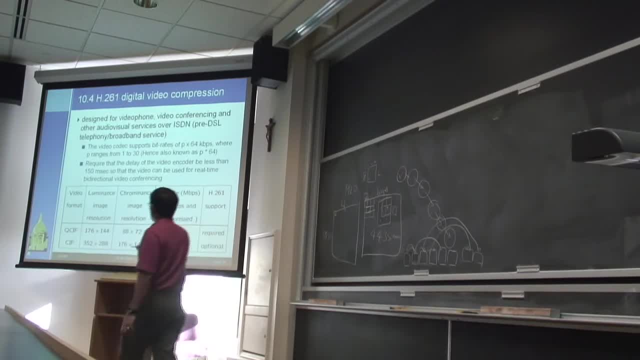 2 is to 0 down sampling. So the luminance is QSIF and the covalence is one fourth of that, which is 88 by 72, right, And if it's uncompressed you'll need 9.1 megabits per second. 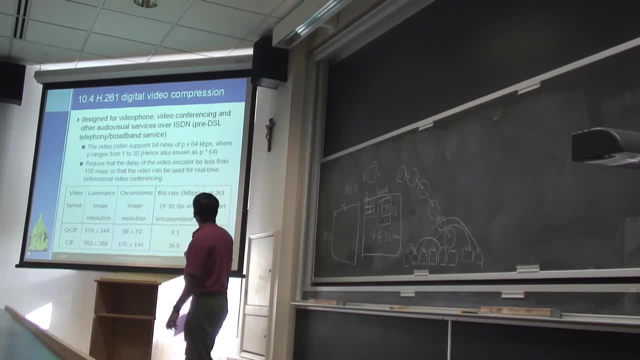 And obviously you're trying to send it through 64 kbps And the standard required this to be supported and this was optional. SIF was optional, QSIF was. QCIF has to be supported. I think they built few video phones like this. 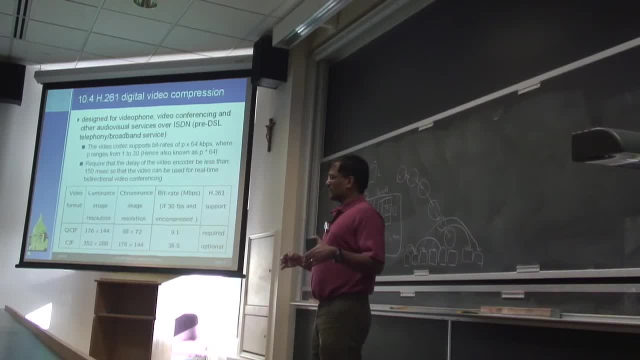 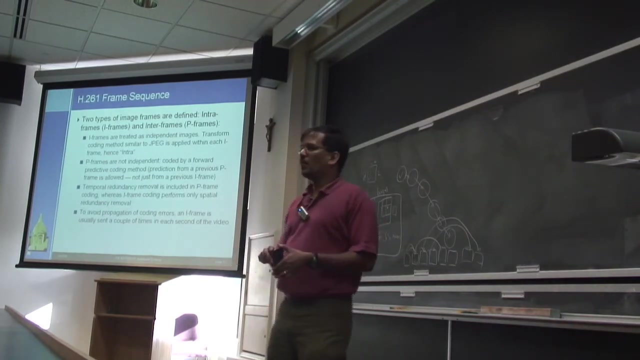 and if my memory serves right, they cost like tens or thousands of dollars. So many people couldn't afford $10,000 video phone on their homes. But regardless, the technology they developed was useful. So they introduced some ideas which we still hold on to. One is the notion: 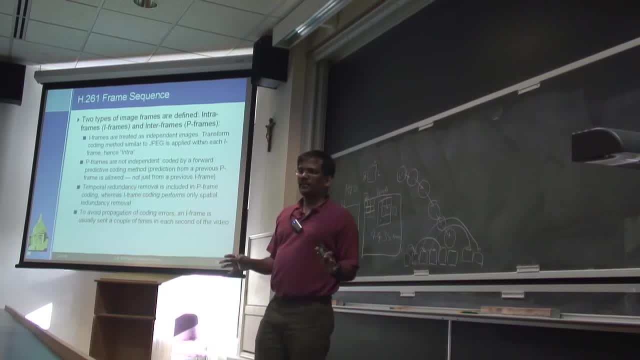 of the intra-frame and inter-frames, I versus P frames, And this is more of a modern concept. And they also introduced the notion of macro blocks, where you have these blocks but you kind of club them into larger group of blocks that you operate. 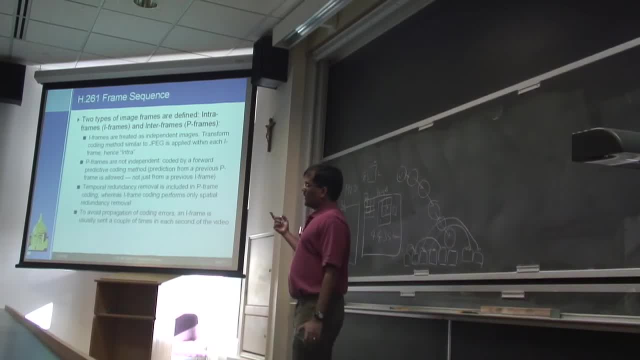 on rather than just on a block, And you'll see why that is needed. because you could, if you define so. one option is to say: let's say this is the size of a block, So I can define this as 4 blocks. The notion here is: I may club. 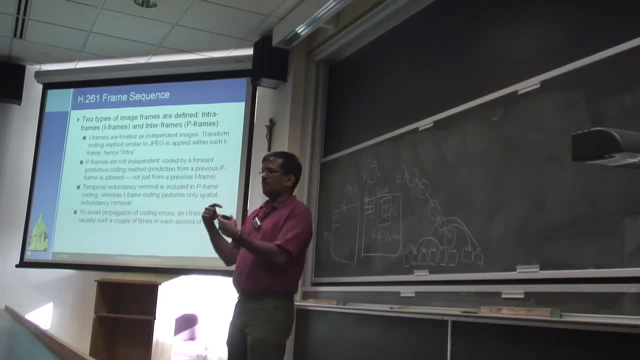 these 4 into a concept of macro block, which is essentially a 2 by 2 matrix of blocks. The question is: why can't I just define my block to be that much bigger? The reason why you don't do that is when you do this down, sampling your luminance. 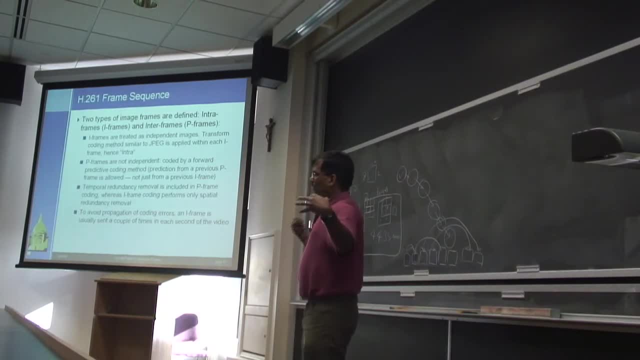 may be in a different size than your chrominance. So you want to make sure that all the computation happen on a block size. So your luminance may be operating on 4 by 4, because it's 4 to 0. Your luminance is 4 times. 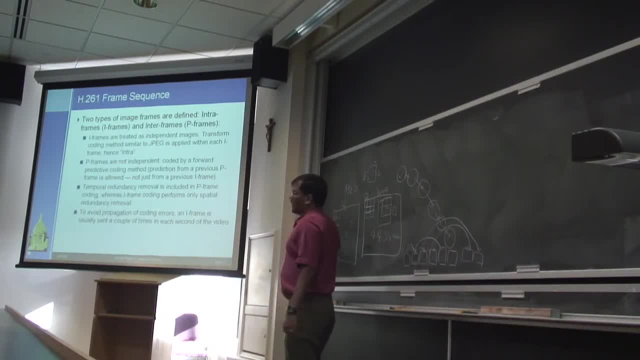 your chrominance values. You may operate on 4 blocks, which you call the macro block. At the chrominance level you only have to operate on one block. So you need the notion of something and one fourth of something because of this sampling. So they introduce: 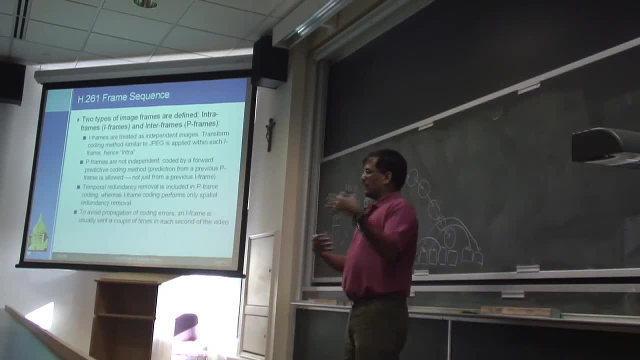 the notion of a macro block and a block, because when you operate on different luminance and chrominance you need different sizes. So all these algorithms work at least on the size of a block. For luminance, they operate on a macro block, which is basically 4 blocks. 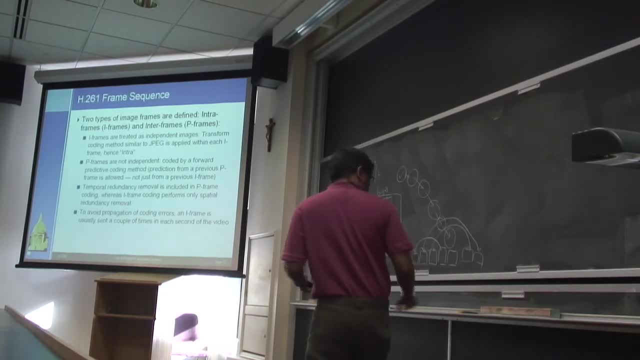 So the main thing that they introduce, which sort of seems obvious at this point, is the notion of an I-frame and a P-frame. So what they do is the goal here is: some of them are called I, some of them are called P. So you have. 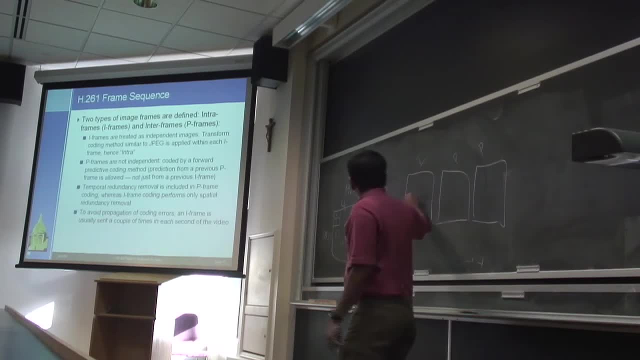 multiple frames that you want to transmit. So I-frame is the base frame and then P-frame is the predicted frame. So essentially, using this, you predict something about here. So you use this one and then you can do a motion vector and say: this frame is generated. 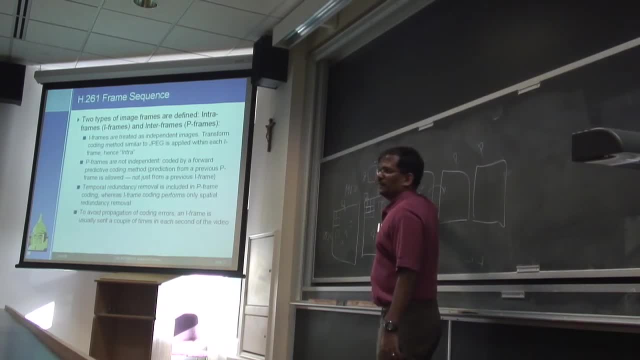 in software. So essentially you have to transmit this frame and once you have this frame, this one is built based on here. It may be built as you take a copy of this and then you do all the motion vectors, diff vectors, to see how they differ. 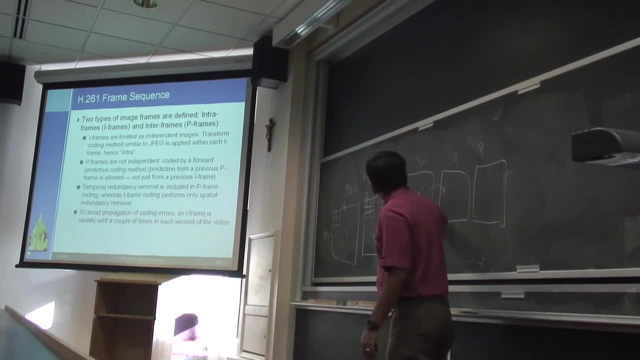 So if this frame and this frame things only changed, let's say around here, So essentially you can make a copy of the whole thing, Then something here will tell me which of the blocks have to be translated from somewhere to the motion stuff and which of the differences I have to do. So 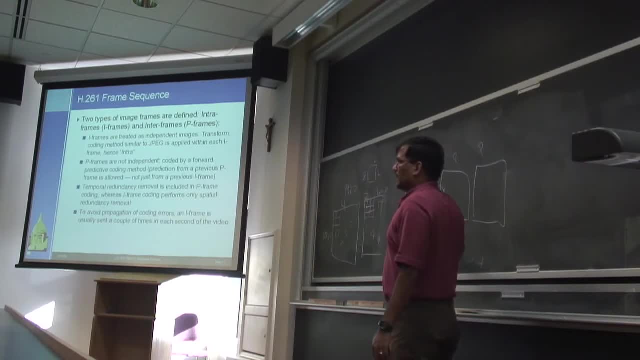 I calculate this frame on the receiving end when I'm decoding based on this frame, Right? So I is the intra-frame and P is the inter-frame and P is forward predicted from the I-frames. Does that make sense? This is a way of articulating what we were doing before. 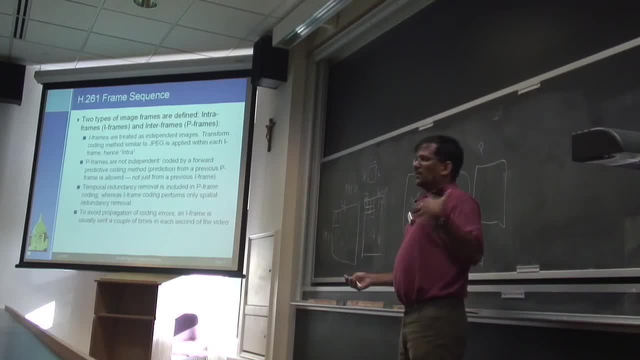 So the compression algorithm was predicting something from the past. so we have to say there are some frames which are independent by themselves. They don't depend on anything else. The predictive frames are dependent on this one. So when I'm transmitting this stuff, when I'm sending something to you, 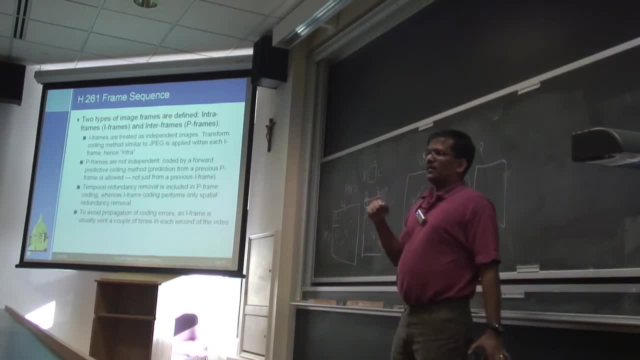 you know which frame is what. So you know that if I get an I-frame, that is so you can do whatever you want on the I-frame to get compression within that I-frame, because you can use a special, you can use a JPEG on the I-frame, Right, But the 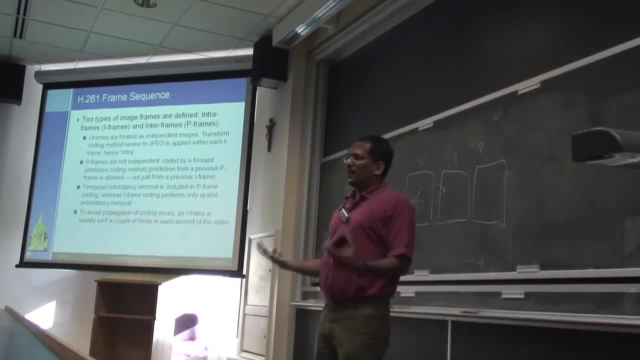 I-frame would be as it is When you receive it. on the other end, it will be as it is- The P-frames. you would have to have your prior I-frame and you're computing this on the fly. So when you're decoding this stuff, you need this frame to calculate. 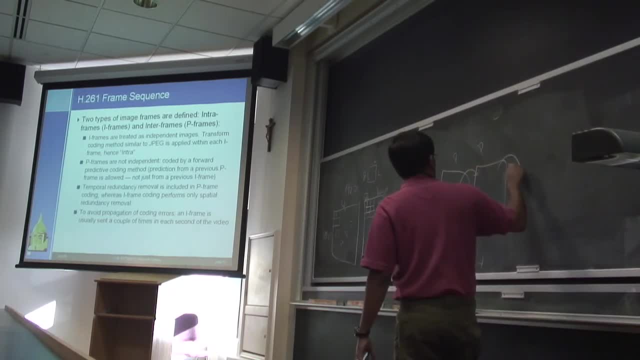 this stuff Right, So it may happen that I can. I may have multiple P-frames to generate this stuff, Right, And at some point I may have another I-frame Right. It need not happen like this, So you may be able. 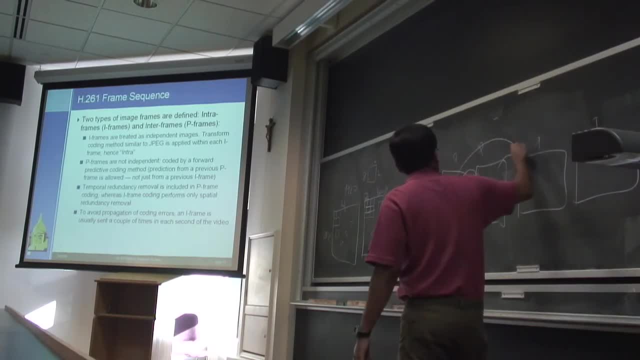 to. instead of predicting from here to here, you may be able to predict like this Right. Basically predict this one based on here Right, In which case it may be like this Right, Which is based on the I-frame. I predict this frame and based on this. 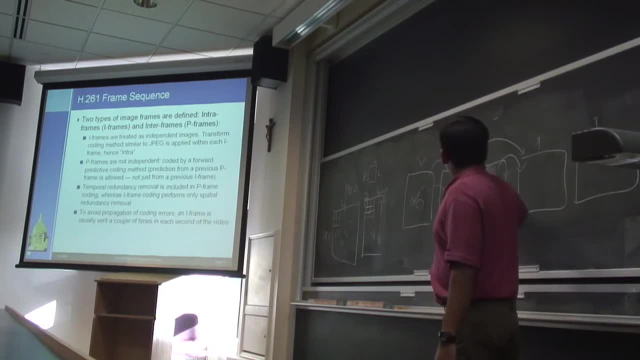 frame, I predict this frame and based on this frame, I predict this frame. and this may not exist, Right. So there are complex ways of saying this stuff. Essentially, all of them are forward predicted. In the future we'll see how we can do backward prediction- Same idea, but 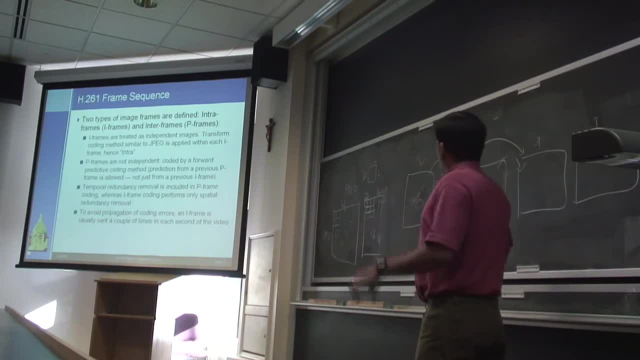 so essentially you're doing this stuff Right. So now that the I-frame, you have to just compress it like a JPEG or something and then you're doing all this stuff Right. So can you get away with one I-frame for the whole video. 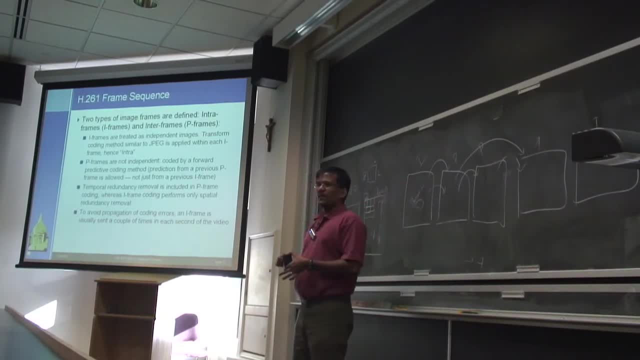 I had another I-frame over there, Right, Why would I have more than one I-frame? Yeah, If you have a scene change, then motion estimation would be very bad. Yeah, so the scene may have changed such that. so ideally I would like the I-frame to be the start of. 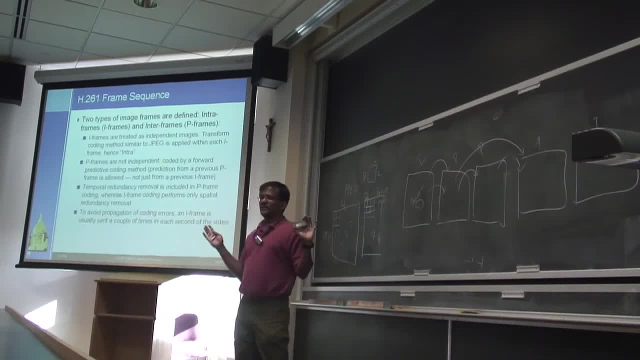 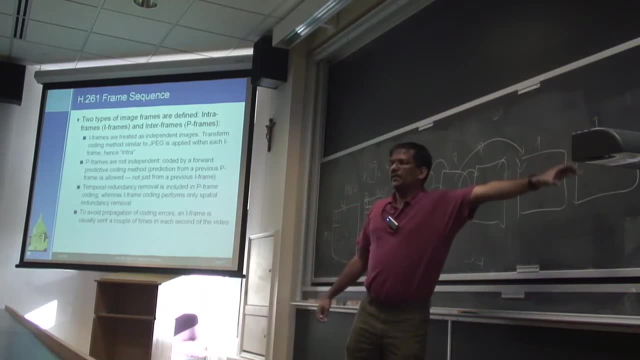 a new scene, Right? So if I can know that in many cases it's not as trivial as it sounds, but if I can know that, I can predict that this is a new scene and that's a new scene, Right? So all the forward predictions for the next scene. 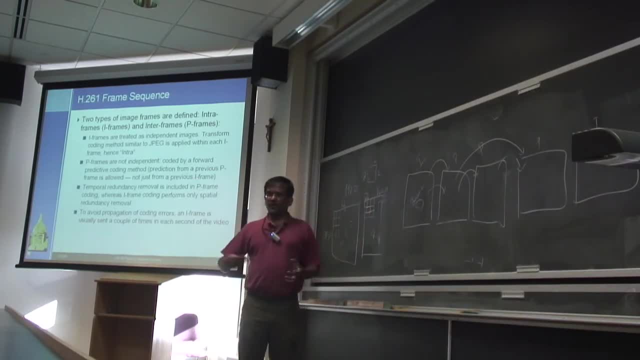 should be from the I-frame, because otherwise you're going to be, you won't be able to predict, because things change Right And it may not be true all the time, because scene change is very hard to detect, because scene change is not necessarily as clean as you want it to be. 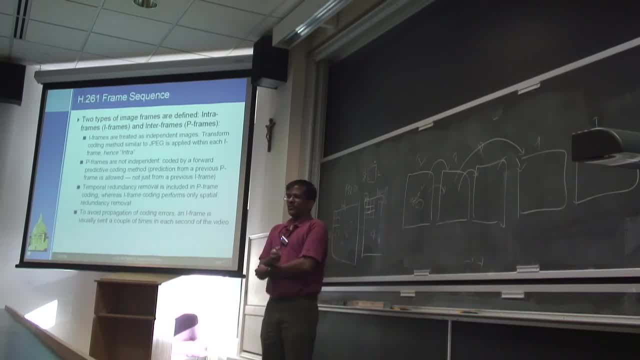 but that's one reason, Right? Is that the only reason why you want the I-frame to a new I-frame? Yeah, It would make the next couple predictions a lot easier. So the prediction right after the I-frame is going to be a lot. 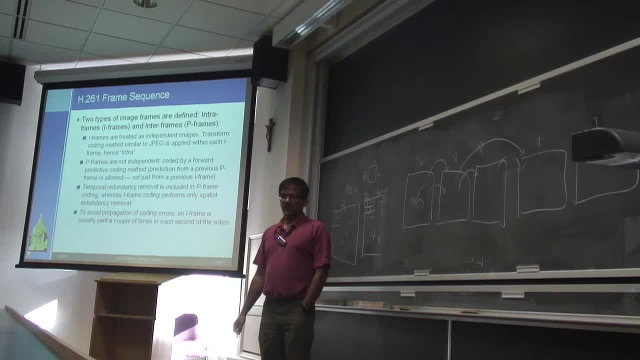 easier to do than a prediction a bunch of ways. Yeah, exactly, That's an excellent point, Right? So imagine, if you have a picture of the quad, Right, Let's say, we have a picture of an upward dome, Right, Not quad, just a dome. 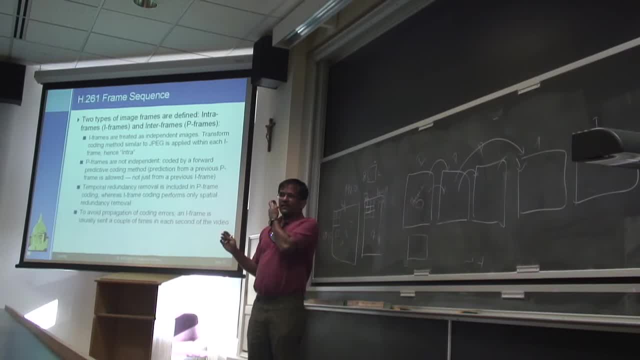 Assume there are no birds and stuff, Right. So you're just looking at the dome, Right, So nothing really changes for the most part, Right? I mean, the dome is not moving, The camera is not moving, You're watching at the dome, Right. 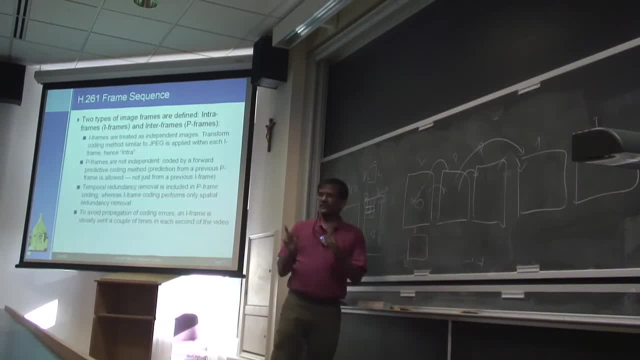 So I can do a prediction where I can have this I-frame as the first. so let's say, in the morning 8 o'clock I start this stuff, Right, And I can use that all the way till the evening, Right. But even though I could use it all the way, 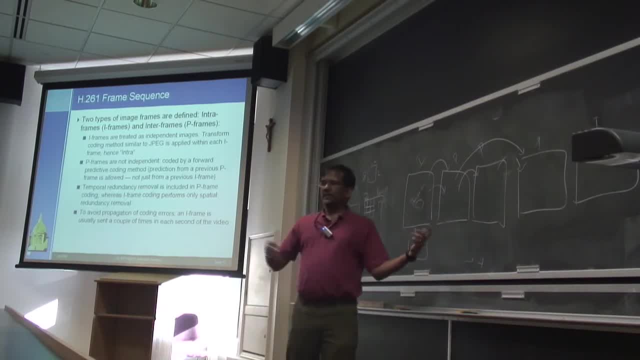 till the evening. Right, The things do change. I mean, you know there's sunlight coming in and then evening changes and all those things. So there are shadows and stuff which are kind of changing. So you have to predict all the way for a few. 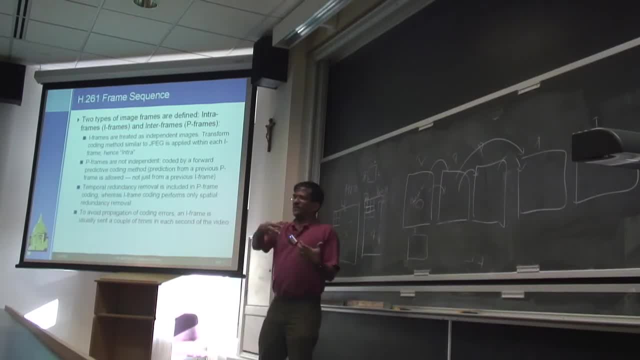 few hours, Even though things don't really change all that much. the computation may be kind of expensive Right, And so it may be good to kind of check point at some point and say you know, morning time it's all fine, but when things 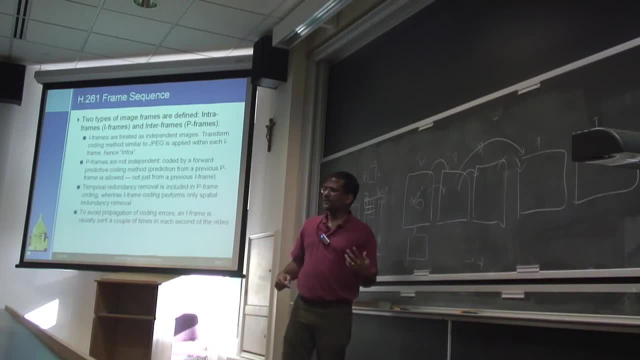 radically change. I would like to have more I-frames, So that's another reason why to have more I-frames, Right? So are there other reasons why you want to have more I-frames? Think of this as a transmission thing, Right? 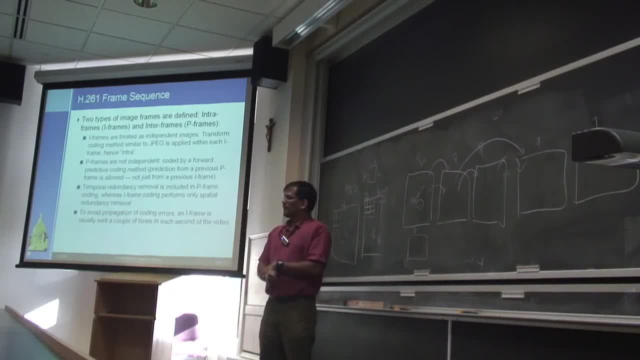 If you are transmitting this, how does I-frame play a picture role in how you view this stuff? Right, Let's say, this is how your TV is broadcast. Right, Does that make sense? Yeah, Would it help keep the quality at a certain level? 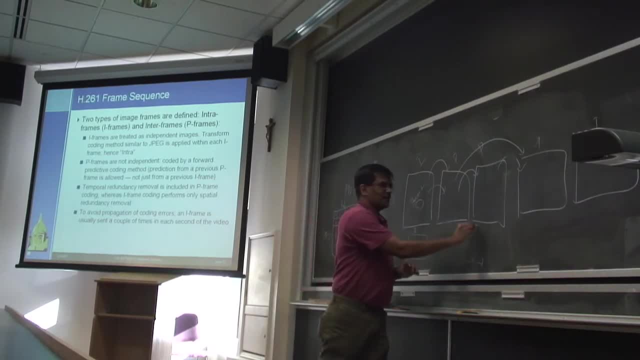 Yeah, more weirdly if I come. so let's say, this is being streamed, Right, If I come in at this time, Right, Can I watch this stream. I need this I-frame. Right, I can't do anything till the next I-frame, Right. 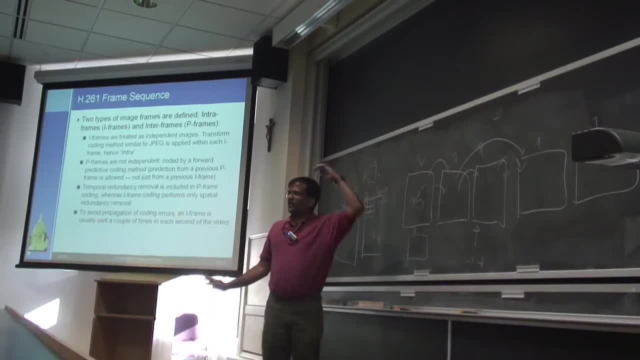 So I-frame is independent, Right. It tells you all that is needed and then all the prediction happens from that stuff. So if you start in the middle, P-frame itself only predicts from what happened before. So unless you have this stuff, unless you have a way to get that back, Right? 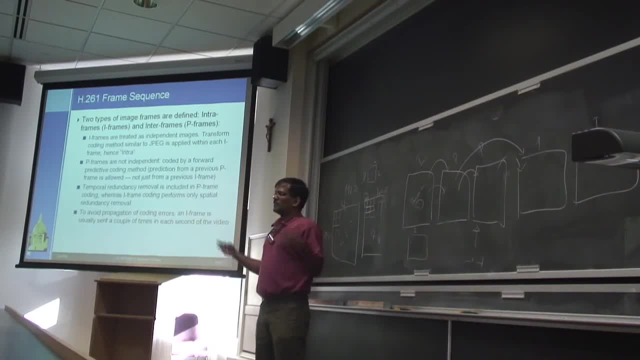 So you may be able to get it back. you may be able to do it depending on the technology. So if you are talking, let's say, a DVD or something, it may be able to go back. Right, So you may have noticed this If you are playing a DVD and stuff, Right? 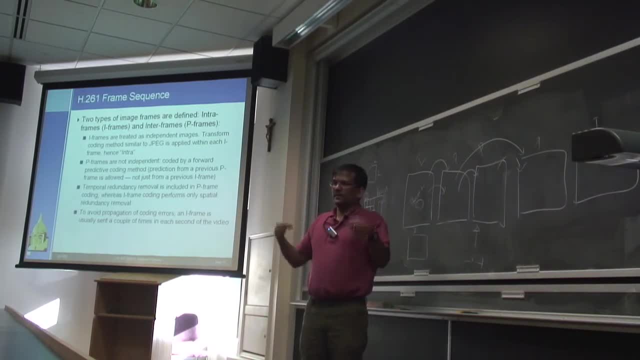 You can't exactly stop and play from wherever you want it, Right? If you say pause, it sort of would pause after a little bit. Right, Because you can pause watching where you want, but you can't start playing from this frame. Right, It has to start playing. 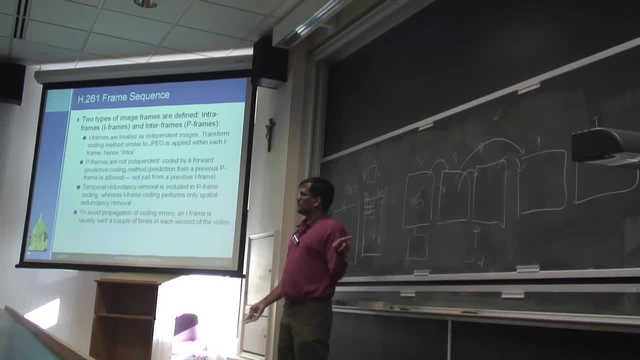 from here, because I-frame is the one where it starts processing, Right? So if it's a TV being broadcast, if you are again looking at the dome, If you are doing one I-frame in the morning and then nothing after that, Right, Then if it, 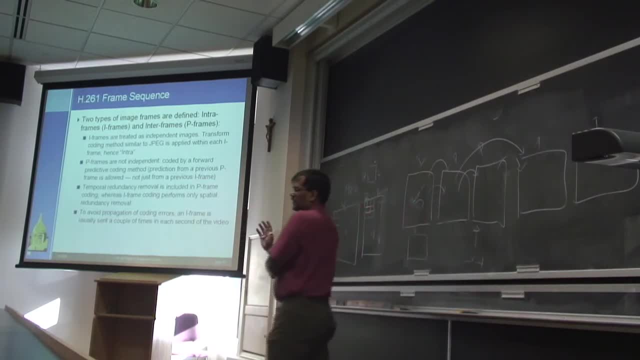 anybody who comes here would just be seeing P-frames, so they don't really get to see anything, Right? So you want to have more I-frames because you want robustness, Right. So there are a number of reasons why you want different I-frames. You want it because when there is 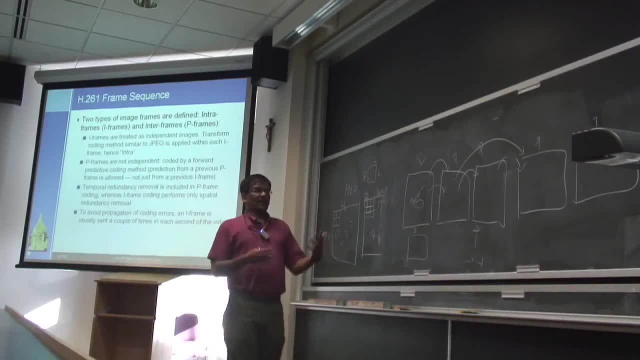 scene change. if there is not a scene change, you want I-frames, And when there are no scene changes, you don't really need an I-frame for the compression algorithm, except if it's like too long Right, Like take an example of a dome. 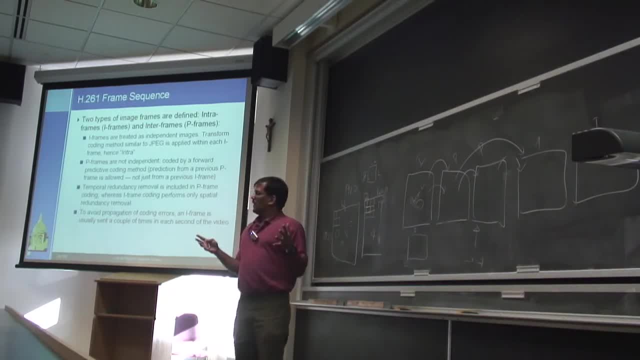 But even within the, when there is nothing really changing, I would want to send an I-frame once in a while, because otherwise you will. you won't be able to join the system, Right. So that's the challenge. So I have to figure out what. 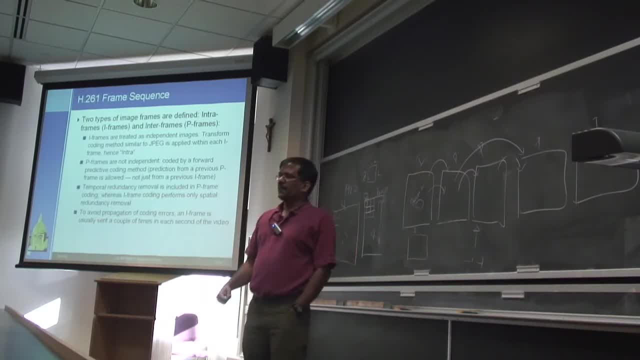 how many, how often I should send this I-frame, Right? So what's the reason why you wouldn't want to send lots of I-frames? Would you want to send I-frame, every frame, Right? Yeah, That would be stupid, because then you wouldn't even get any. 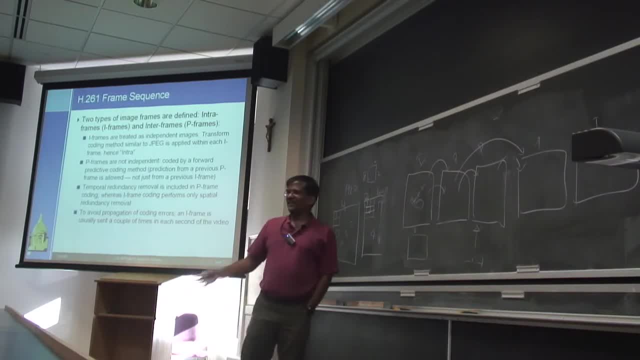 benefits of the Yeah Yeah, If you send an I-frame every time, then it essentially becomes a motion JPEG or something. I mean you're doing JPEG every time and then you lose all the stuff, Right? So the trying to figure out where this number. 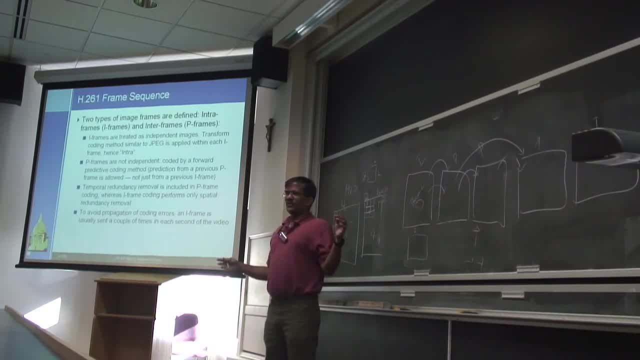 should be is an art, Right? It's not a well understood art And it mostly happens based on image analysis, Right? So when you're doing a project, you'll notice that systems will ask you: how often do you want the I-frame Right? 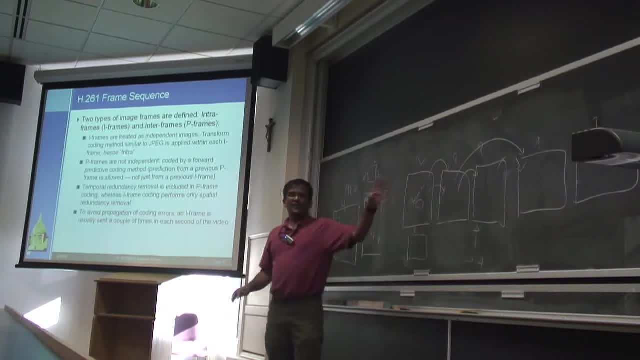 They don't ask you about whether P and most of the modern ones also have a thing called B, which is bi-directional prediction. We'll see in the future, Right? So essentially they don't care about how much this stuff, but they want to know how often you want to have it. 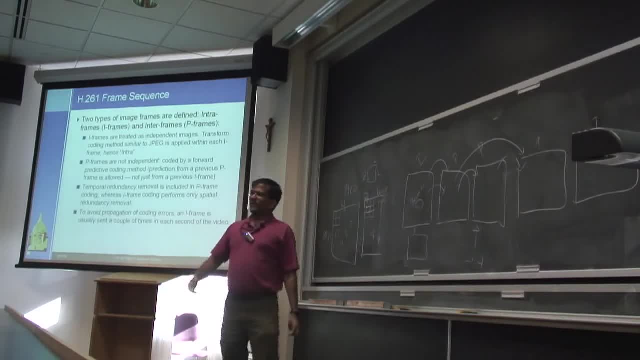 Right? So it's simple to say you should have I-frame every so often, Every 30 frames or what have you Right? But what you really want is the stuff we discussed. What you really want is, whenever there's a scene change, I should have I-frame. 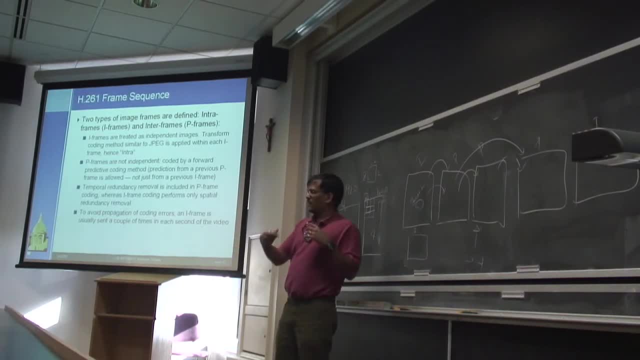 and otherwise. I should see how far ahead you have gone to intelligently decide where things should happen. Right, And that is very computation intensive and that's one of the reasons why the thing I was talking about takes that much time, Even though in this particular case, 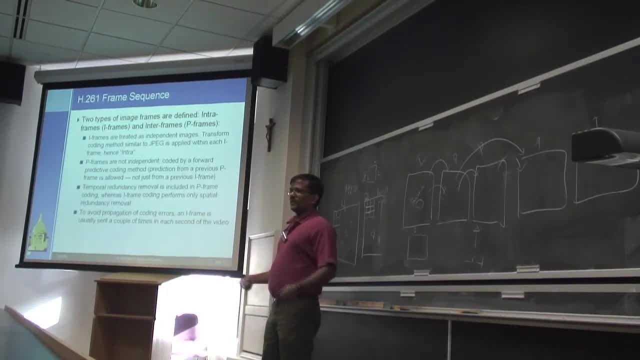 the only thing which is moving is me and this screen. the computation algorithm is very hard to figure out where the scene changes and where to put that I-frame Right, And you want a good balance, because if you don't, then so I-frame tends to. 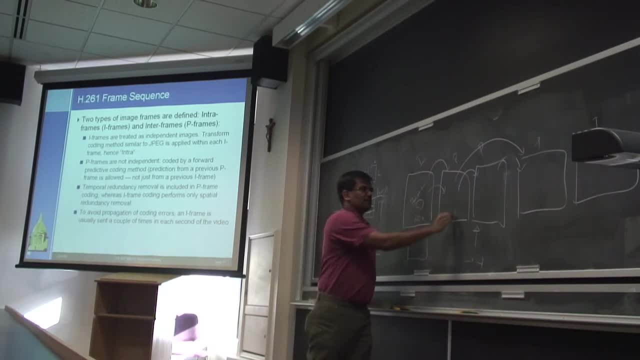 be, let's say, about 20 times as much as these frames. Right. Again, it depends on what you're trying to see, Right? So if this happens to be able to be predictable, so if I'm looking at the dome, you can possibly have this as 0x, Right? 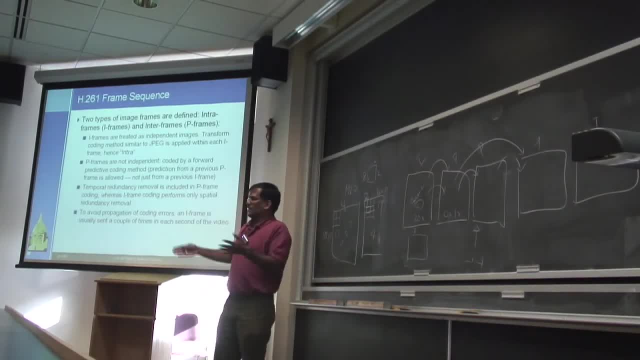 Because the P basically says the dome is where it is and nothing changed, And so on and so forth. So you send the I-frame. nothing else happens after this at all, whereas if things are moving, depending on how much they're moving, you expect this to be a different size. 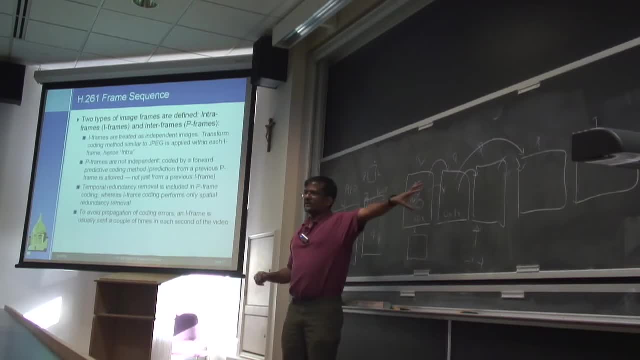 And at some point you may decide that if this and this have sufficiently changed enough that the, if the P-frame happens to be, say, 15x, Right, Because there's so much motion from the previous one, You may decide to say, well, I don't want this. 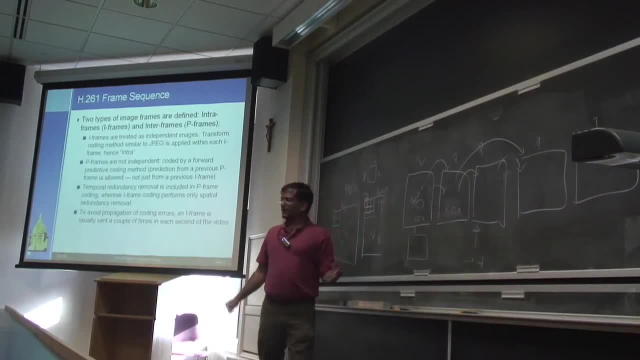 I just want to send the the whole P-frame because it's changing so much, so let me send the whole thing up, Right? So that's a dead man call from you. So, depending on how these scenes or things are playing out, this will always be big. 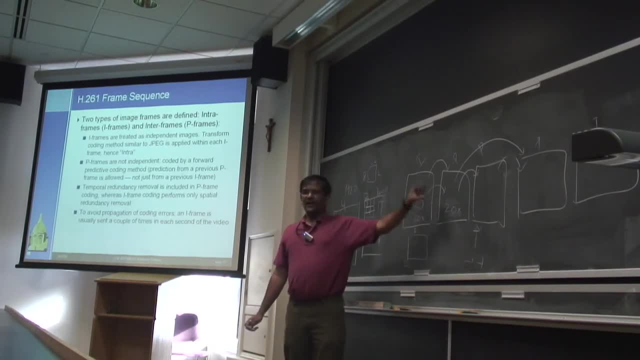 Right, Because this is compressing the whole image. This one can be can be variable, Right? You don't want it to be go to ever go more than 20x, Right? So if the prediction happens to be that, the prediction is like 40x size, 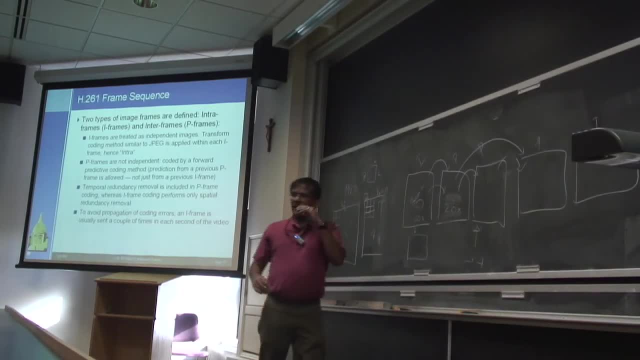 Right, Then clearly you don't want this. you just want a new I-frame, And that's a challenge. Right, Thinking of how, what this means for our transmission, Right, Our transmission, or what you do with the systems, Right, Once you do this compression. 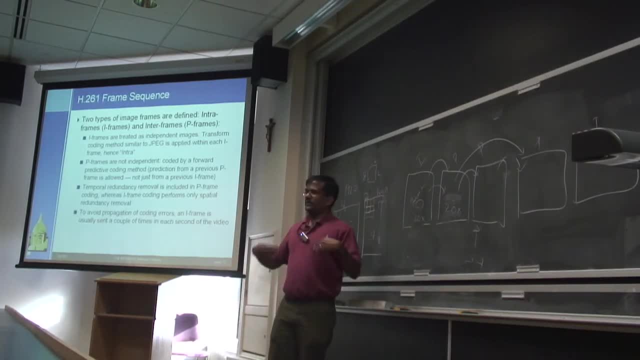 even though I talk about I-frames and P-frames, when you are transmitting it on the ISDN line, Right, I may talk about it as every 1 thirtieth of a second. I want to send a frame because you know I expect you to show. 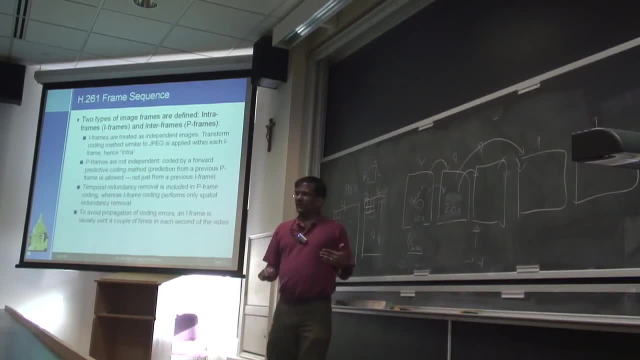 30 frames per second. so that's what I expect, Right? But what would that mean? for on the wire, You need 30 frames per second, Right? So I have 30 frames here, Right? And let's say, for ease of description: 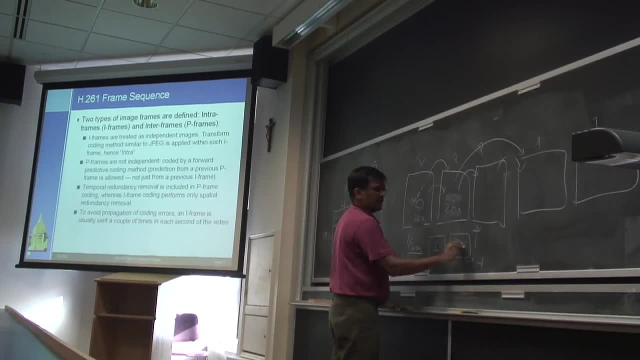 I have one, I and I have 29 P's Right. Right, And again, for ease, let's say, this one takes 20x and this one, each one, is like 0.5x or something, Right, Some small number, Right. 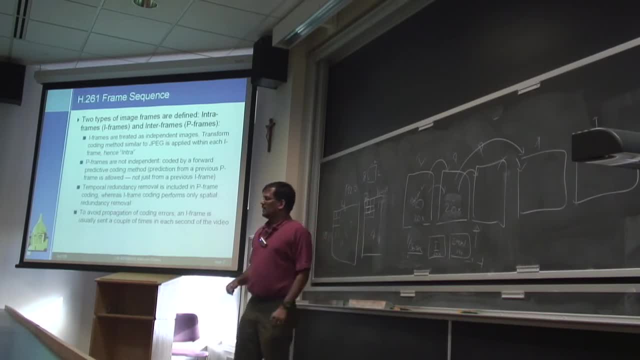 You need to make sure that they all add up to 1.. Right, So some small thing like this, Right? So how would this be? how would this be on the wire Right, The I frame being the bulk of this stuff within the 1 second it's going to. 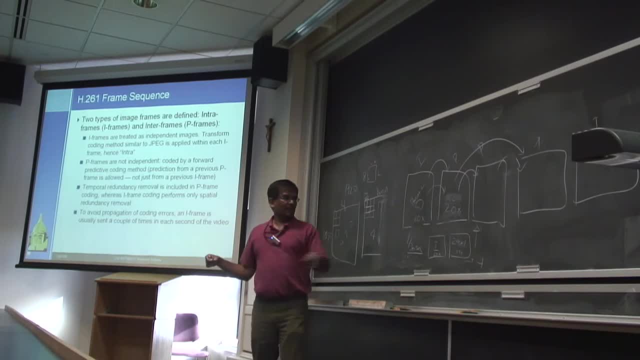 take most of the bandwidth. Right, The P frames tend to be small because they just add something to the previous one, Right. So in terms of transmission. so life was good. if I can say, I am going to send 30 frames per second. so you are going to get. 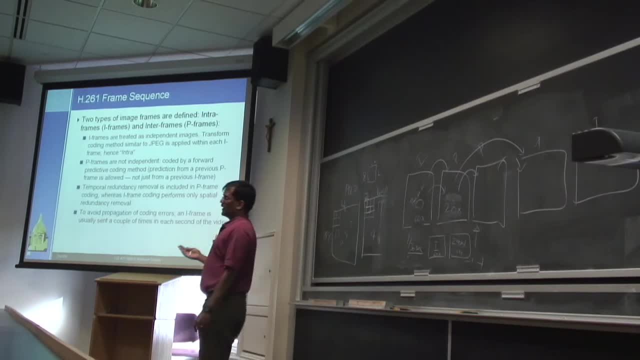 one packet, network packet every 1 thirtieth of a second which you can use it to show it on the screen. but the reality is you are going to see frames which are pretty big and are very important. Right, You can't mess with. 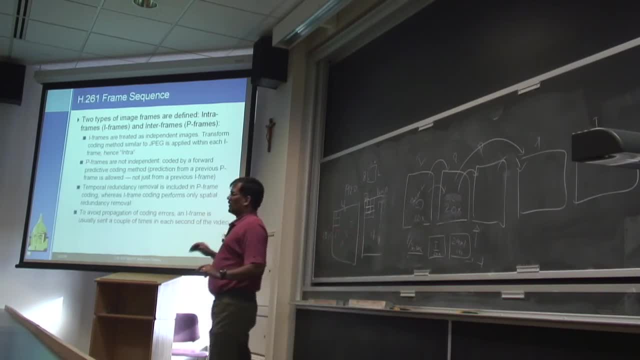 I frame Right. You can lose a P frame and we will see as we move along. you can lose a P frame because if you lose a P frame you lose some prediction Right And, depending on what the prediction is, you may lose that particular frame Right. So in this particular case, 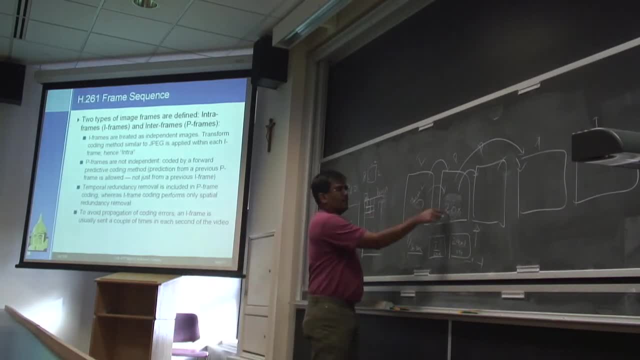 I had you know from I frame, you predict this one Right, And then you predict this one, And this frame was predicted from here, Right. In this particular case, if I don't receive this Right, Then all it will happen is I will have 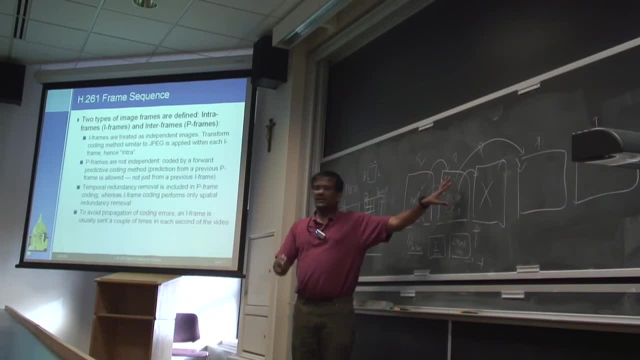 frame 1, frame 2,. I won't be able to show frame 3 to you because I didn't get this information, but I can show frame 4 because it was being predicted from here. Right, If I lose this, then I would lose certain number of frames. 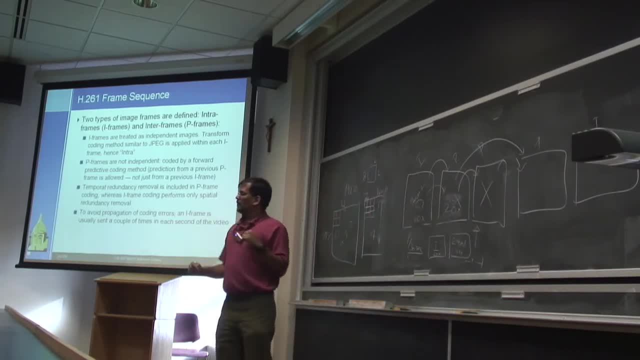 depending on how much forward the information goes forward, But if I lose this, I all this is lost, Right, And so that plays a big role in all the stuff we are going to see. This is the reason why we are going through all this stuff, which is: 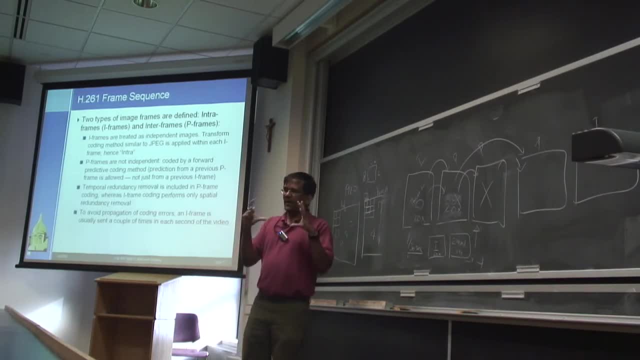 even though we think of video as a big object, it's not a big. I mean, it is a big object. The compressed image is a big object But it has structure which has this weird property that there are some frames which are very important and they tend to be big. 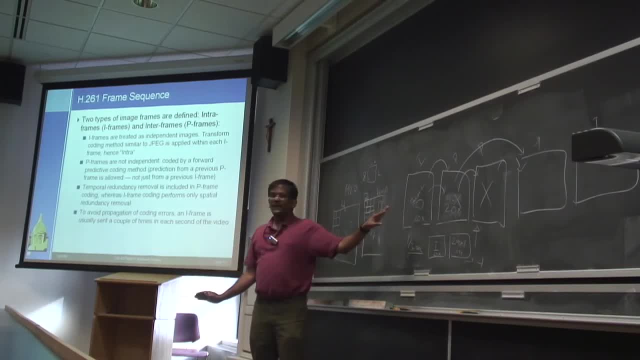 and you cannot mess with them, You cannot drop them. There are other frames which can be dropped Right And, depending on how lucky you are, the effects may be sort of localized Right. And if you don't have enough bandwidth, the 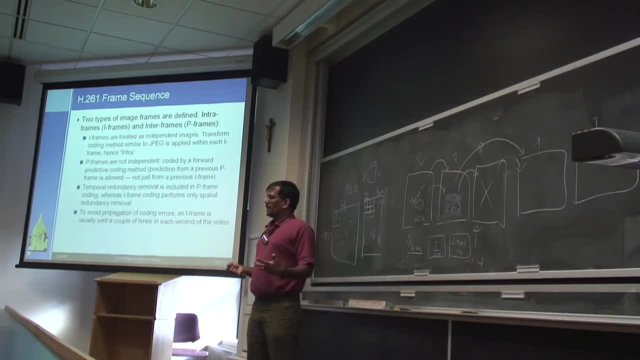 question is: if I don't have enough bandwidth, which frame should I drop, Right? If I have no bandwidth at all? the answer cannot be: I am going to drop the I frame and get all the P frames because they are no use to you, Right? So you have to keep the I frame. 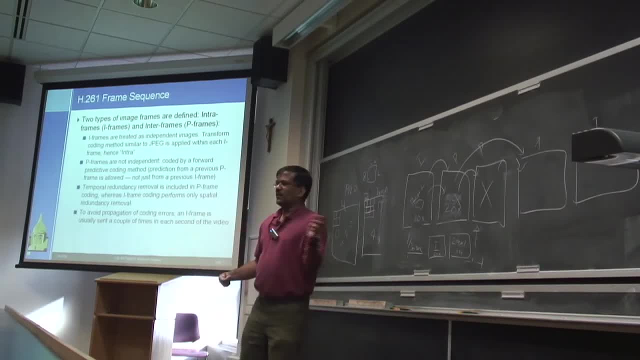 but within the P frame you want to choose the P frames which cause at least somewhat of damage, Right, So you are trying to find out which frames to be sent to you and all those things. So those add complexity. Those add complexity in terms of how to transmit them. 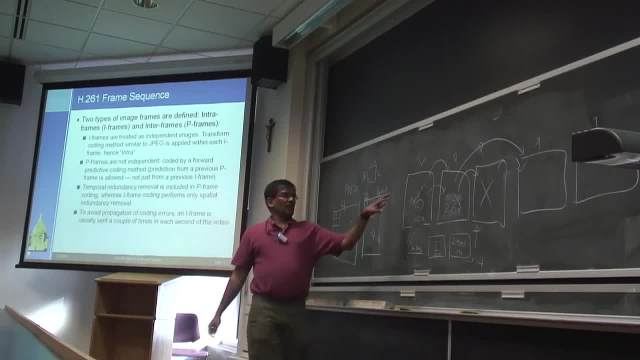 how to store them, how to act with them, and once you get these frames, you have to do certain amount of computation to get these things going, and that's a challenge, Right? And in real life you have I, P and B frame and more complex stuff, Right. 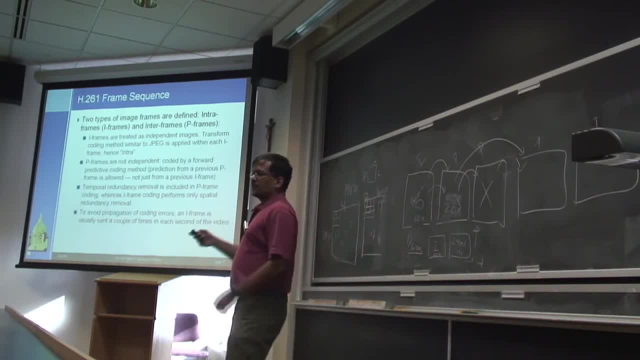 So anyway, so going back to the stuff, So they introduce a notion of I frame and a P frame which essentially quantifies the notion of a fixed frame and the motion vector prediction kind of stuff, Right, So they have sort of like the graph I had. 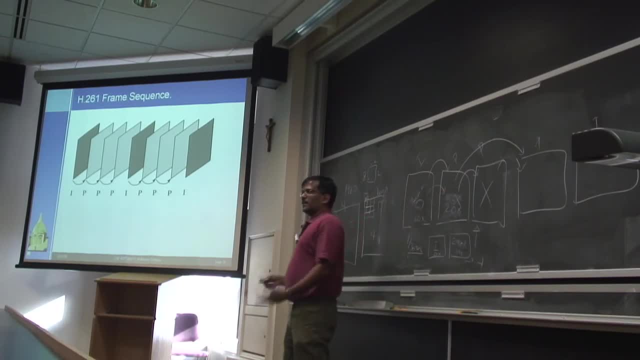 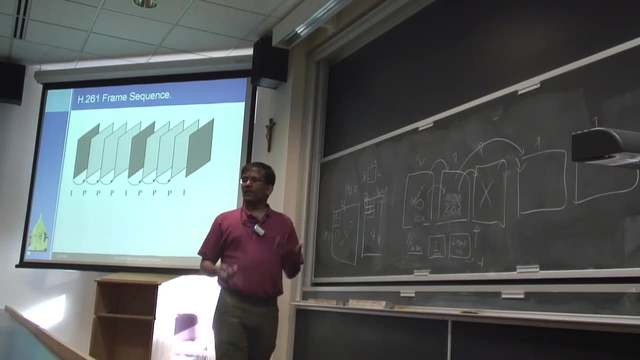 here. So I frames and P frames. The standard does not define how many P frames should be there, how many I frames should be there, And again, that's the stuff you are trying to figure out, and a good number of how much they should be. 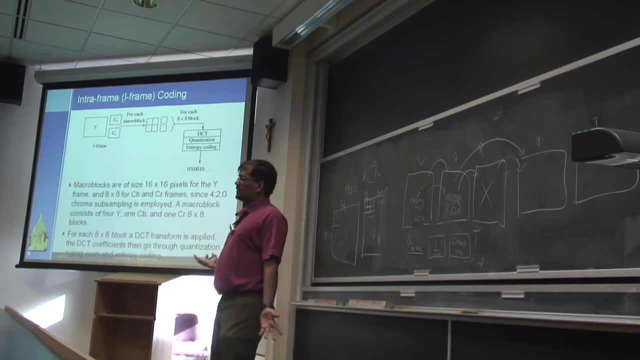 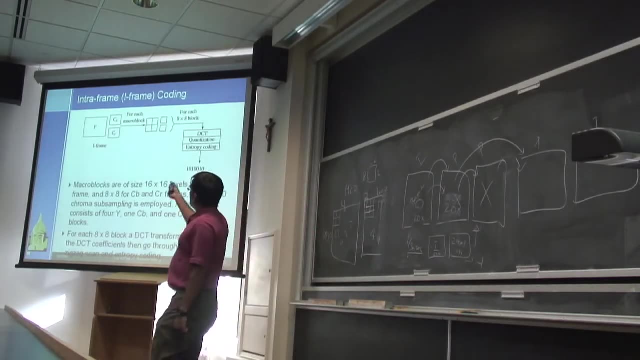 So I frame is. it's no big deal. You know, you can do whatever you want. You pretty much use something like a JPEG compression, Right? So, since we deal with the macro block of size 4 by 4 right, Which is essentially 4 macro blocks in the 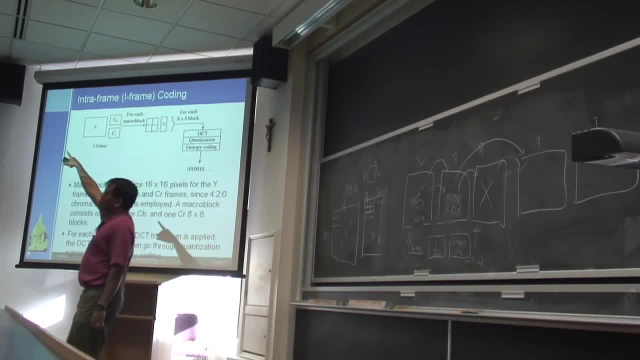 luminous domain like. so if you take the image and do the Y, C, B, C R, right Y would be 4. on the corner Right Y would be 4 blocks. C, B and C R would be 1 block. You generate the macro blocks for them. 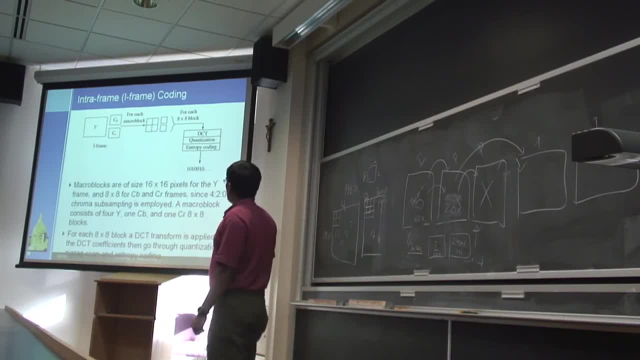 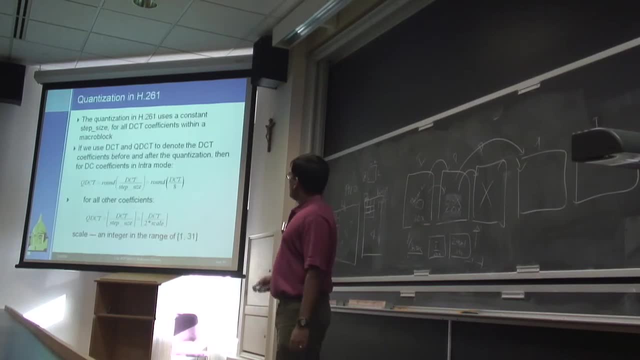 Right. And then you can do your usual multiplicity and quantization and entropy coding Right, The way you do for your JPEG. The only difference is at least in H261 they didn't have the luxury of having the matrices and stuff to do the quantization. 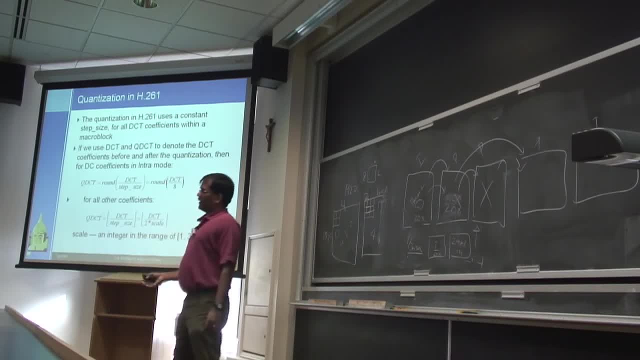 So they simply divide everything by 8 and then simply multiply by 8.. Right, So they are dropping all frequencies equally, and modern encoders you won't do that. I mean they choose some number and use it on all the things I think for the 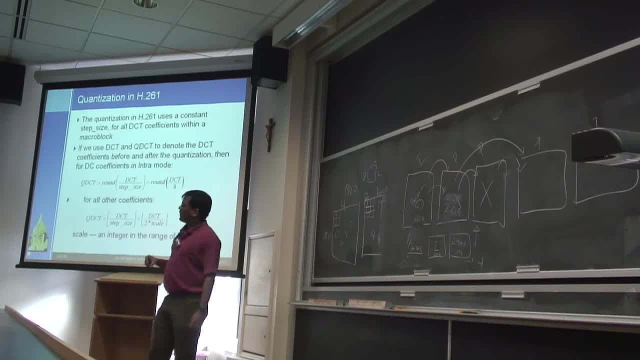 DCT, they drop it by 8. For the AC components they use a different range from 1 to 31. So essentially they drop all the frequencies except DCT at a different pace. But the idea is it's not that different from JPEG. 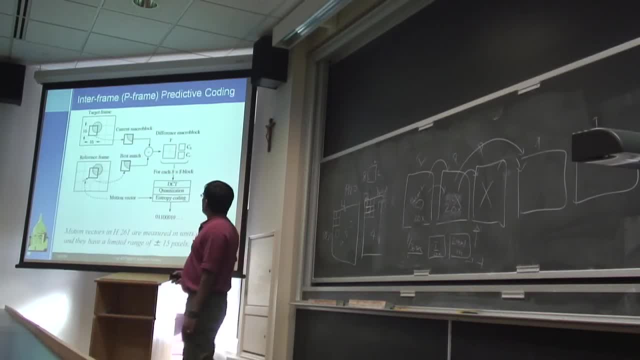 Right, And this they had to do because of the hardware they had. The catch is you have to figure out the. the P frames Right. So the P frame- again you have to. so they only define the P to be plus or minus 15 pixels. 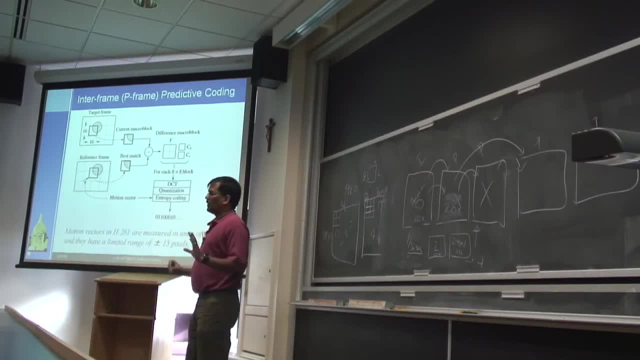 So, from wherever you are, the P is defined to be only that big Right. So you don't have to search the whole frame. So you take the reference frame and the target frame, You do the, you figure out. you figure out what the you figure out what's the best match, Right. 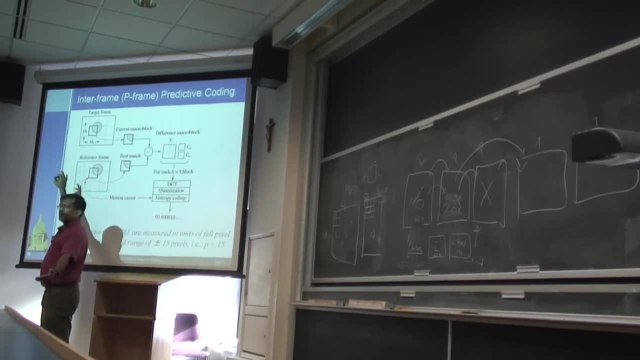 So, essentially, you do whatever You do, the logarithmic or sequential something to figure out where it is in the reference frame And then, once you figure out this is the best match, you look at the difference, Right, You look at the difference between that and the. 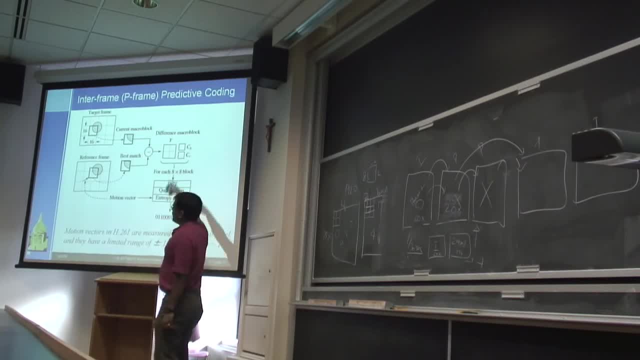 and the one that you're trying to transmit. The difference is too much, Right? So you do a. you have the difference blocks, Right? The difference is too much means there's too much color. Then you may decide that this cannot be really something that you 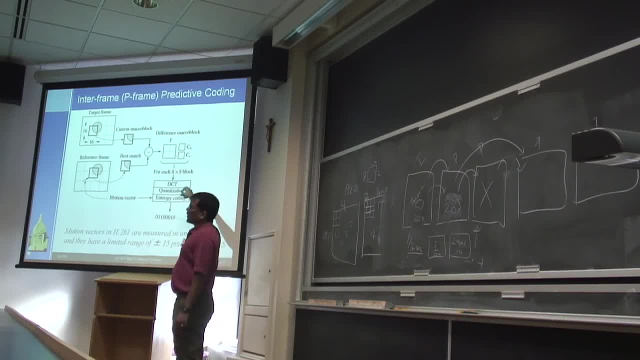 want to look at Right. But if it's okay, then you encode the difference Right. So you encode the difference between the previous from the block from the target and the block from the reference frame, translated Right And hopefully, if, like we saw in the 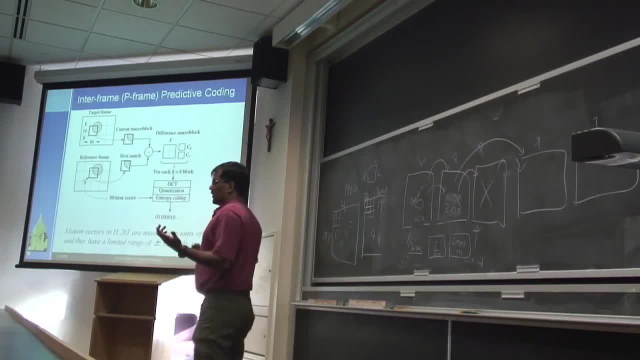 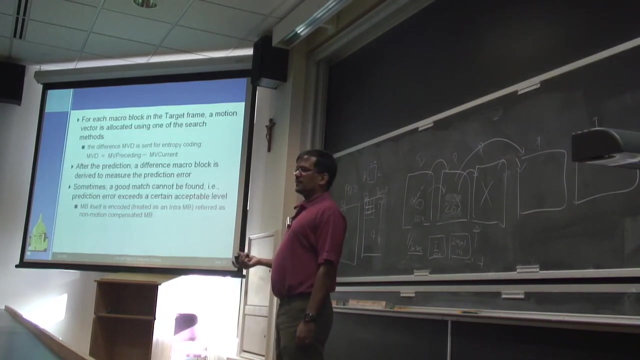 on the illustration it's all black, which means it's all mostly zeros, Which means that there's a lot of same numbers. So this would compress much nicely, Right, And you also do the motion vectors as a difference, Right? The other observation here: 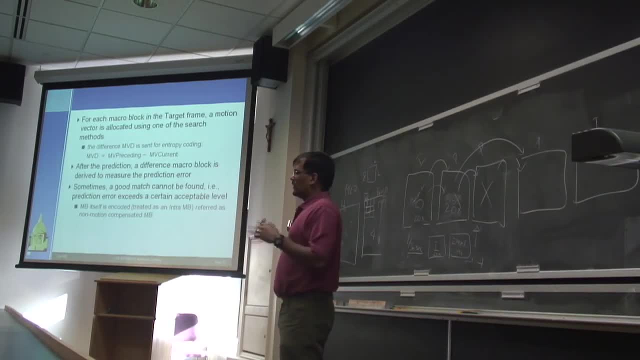 is, things tend to move in the same direction throughout the scene Right, Even though in the example we saw they were not the case. But in general if somebody is moving, then the whole bunch of blocks which are around them, which is going to move in the same direction. So the motion vectors.